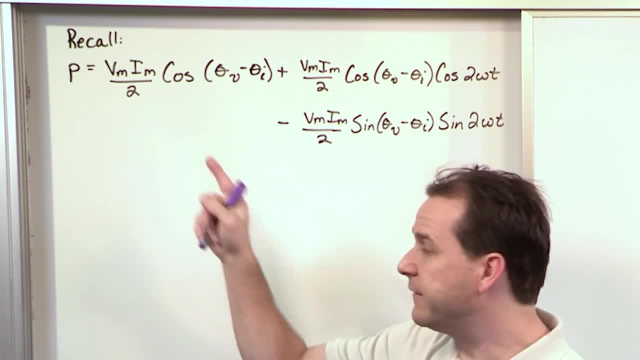 the current and the voltage, which is going to be the current and the voltage, and you be governed by your circuit that you have, And this is going to be some kind of sinusoid over time And it's telling you that the instantaneous power is always changing, But we want to zero. 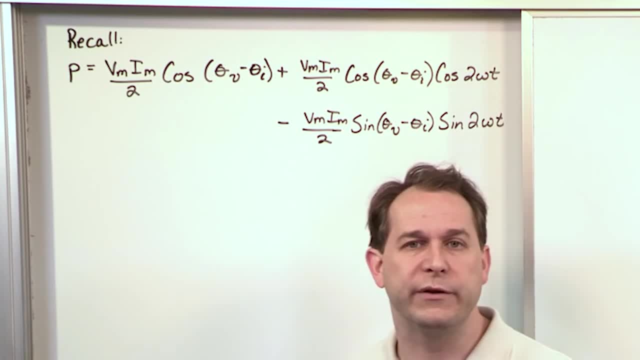 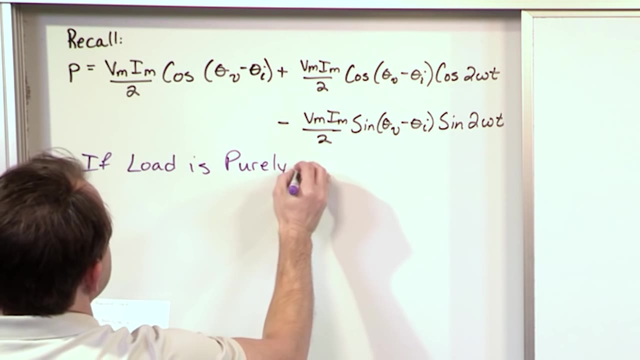 in on the case when we have just an inductive load. What's going to happen when there's just an inductor inside of the box? Last section: we talked about what happens when there's a capacitor in the box. Now we're going to talk about if the load is purely inductive. 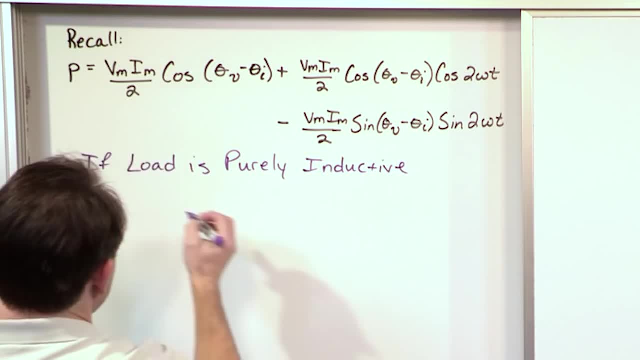 What happens Right now. actually, it's something really cool that happens, And I find this stuff really fascinating with circuit analysis. So this is some of the reasons I'm really excited about teaching it. The first thing you need to remember: there's very, very few things I tell you in circuit. 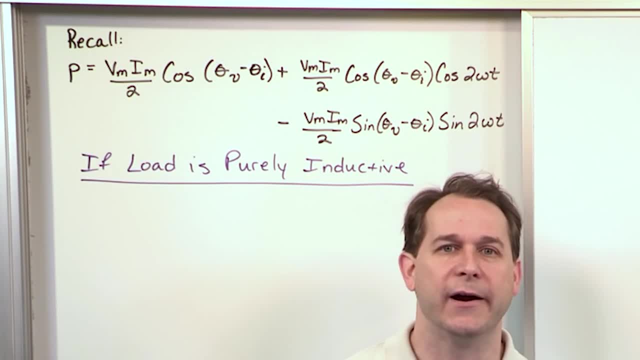 theory. to just remember. One of them is Ohm's law. V is equal to IR. You have to know that. Some of the real basic power equations, just memorize them. What I'm going to tell you here is something you should just remember. When you have a purely inductive load, the 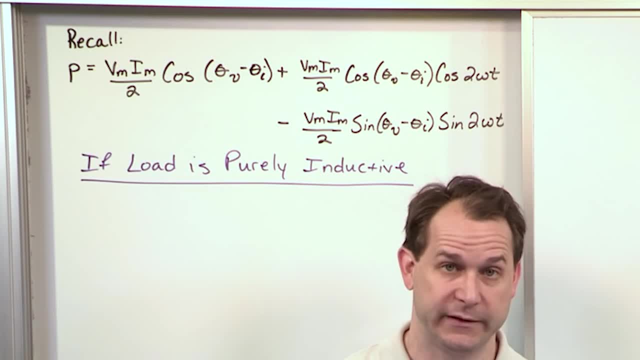 current. Okay, The current of that inductor lags the voltage by 90 degrees exactly. The current lags the voltage in an inductor or across an inductor by exactly 90 degrees. Current lags the voltage by 90 degrees. 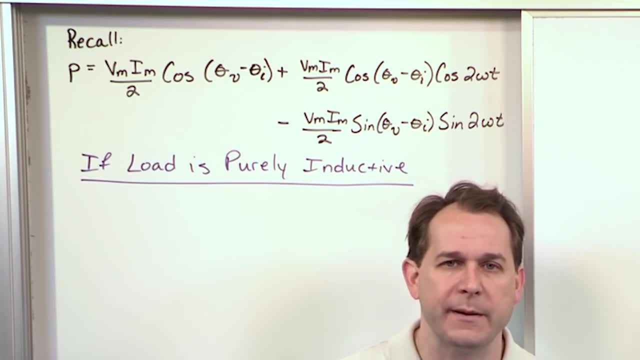 I'm going to show you how to prove that to yourself. but just remember it, Because if you can just remember it, these few little things I tell you to remember, it's going to make your life so much easier. So let's go down here and write that down And I'll explain what I'm talking about. The 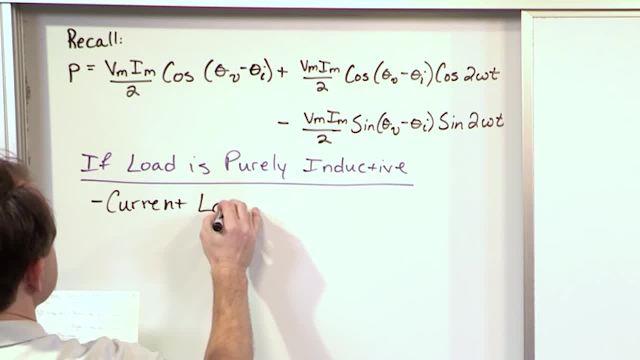 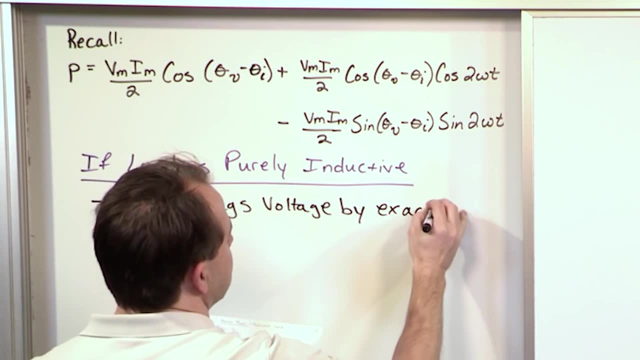 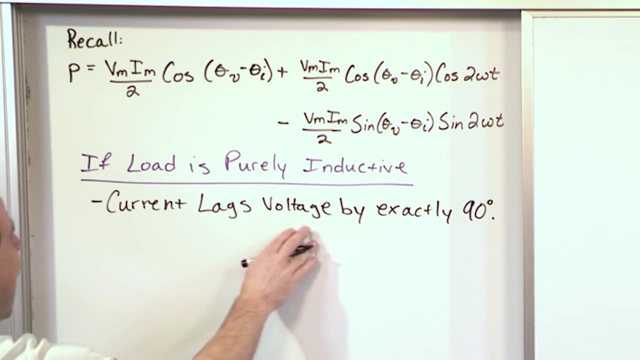 current lags the voltage By. I'm going to put the word exactly 90 degrees, And I'll give you a hint: When we get to capacitors, it's also going to be 90 degrees, but the current is not going to lag. 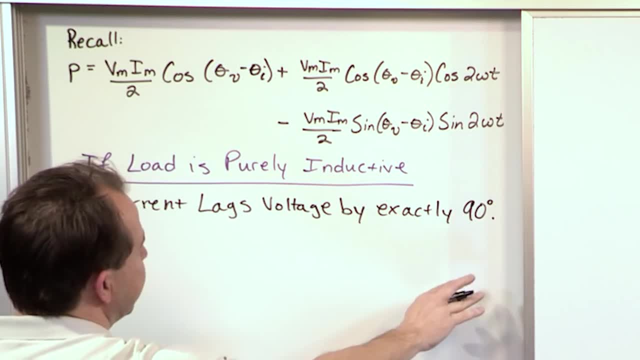 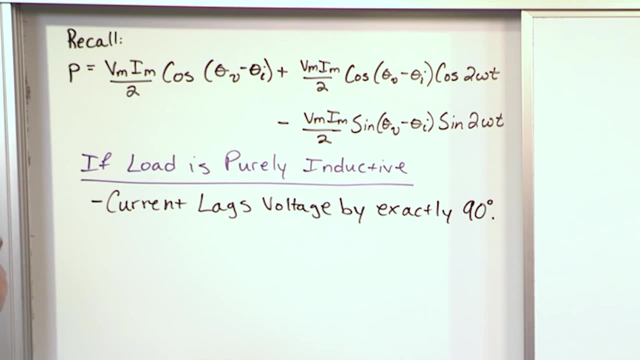 the voltage in a capacitor. The current will lead the voltage by 90 degrees, So the 90 degrees part is going to be easy to remember. The leading versus the lagging is what always confused me when I learned this stuff for the first time. 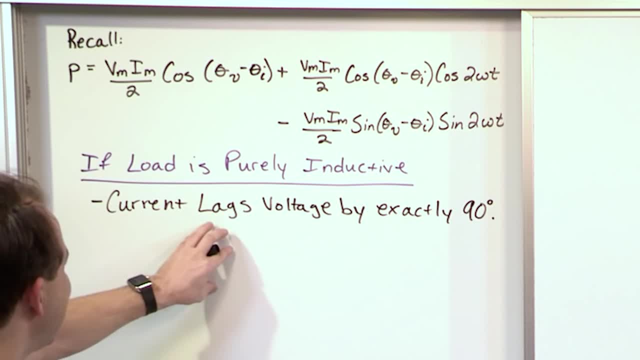 Finally, you're just going to have to commit it to memory. The current lags the voltage in an inductive Or in an inductor, Or across an inductive load, when it's purely inductive. Now why do we care about that? 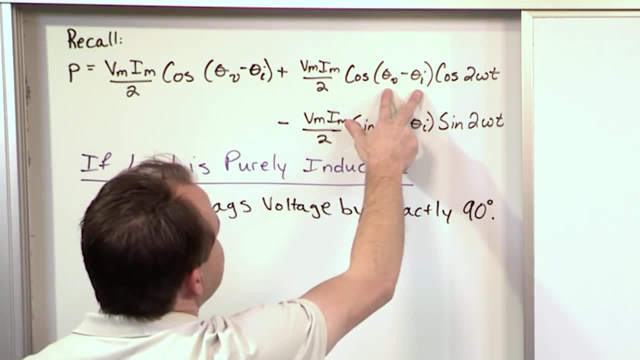 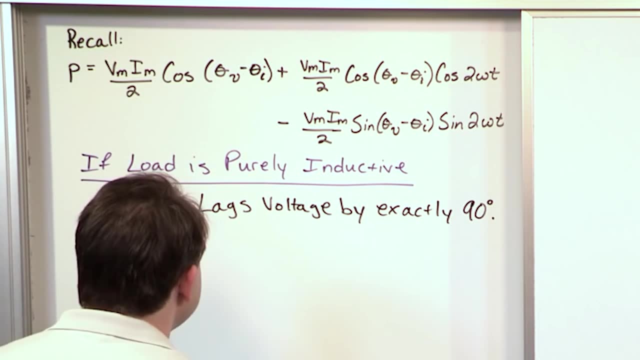 Because in this power equation we see we have all these phase differences between the current and the voltage. So when we say something like the current lags the voltage by exactly 90 degrees. what we're really saying in words is the following: We're saying that the phase 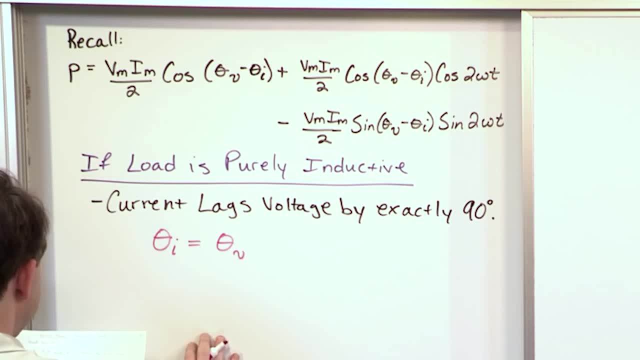 angle of the current is equal to the phase angle of the voltage, whatever it is, minus 90 degrees. Make sure you understand this little equation here. Current lags the voltage. That means, whatever the voltage phase is, you subtract 90 degrees and that is going. 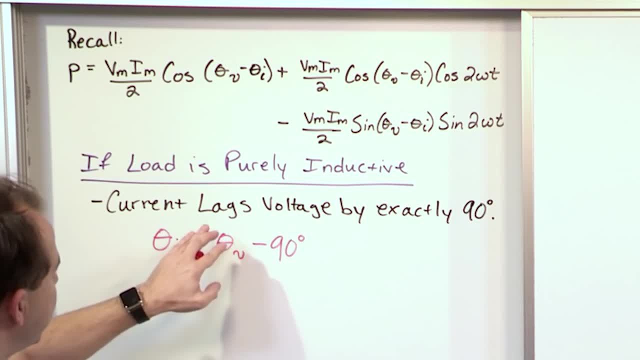 to be what the current is. So again, make sure you understand: Whatever the voltage phase is, shift it 90 degrees, look to the left 90 degrees, so you subtract 90 degrees. That's what the current phase is going to be. So the current lags the voltage by exactly. 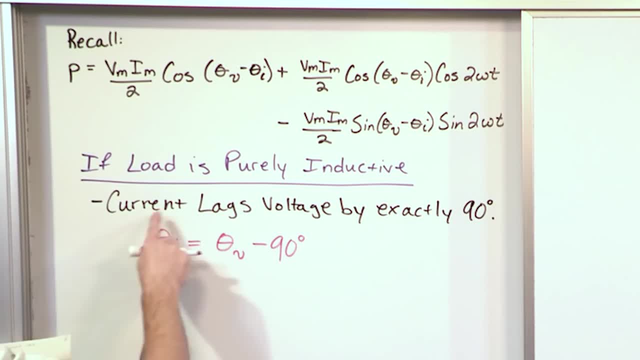 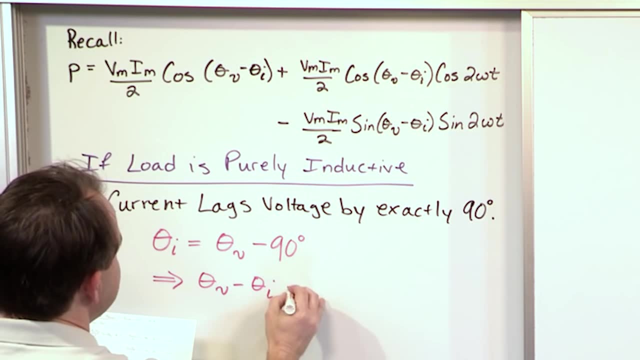 90 degrees. So another way to rewrite this. this is kind of the layman's terms way to put it, but if you rearrange things a little bit, what it's basically saying is theta V minus theta I is 90 degrees. 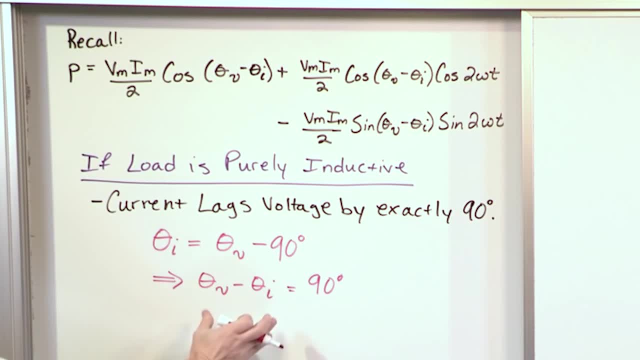 So again, move the theta I over here, move the 90 degrees over there. boom, you get this. Why do we write it like this? Theta V minus theta I. okay, The reason we write it like that- I can even put parentheses around here, if you want. The reason we do that is because 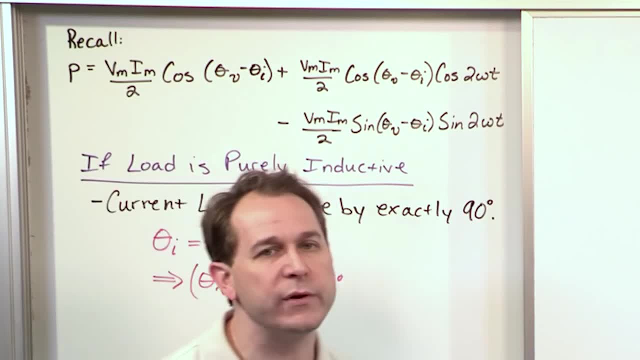 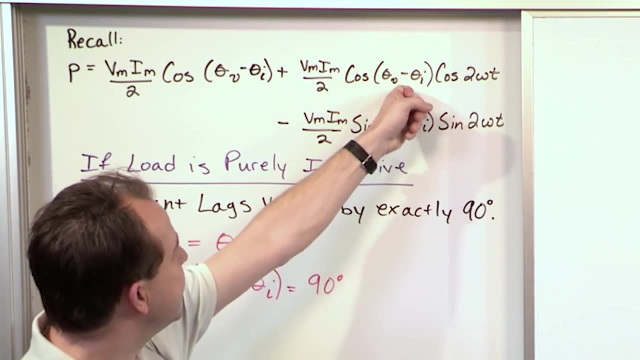 this equation has theta V minus theta I everywhere. So you see, when the load is purely inductive, you basically stick 90 degrees positive 90 degrees in here, in here and in here, And you should know that the cosine of 90 is zero and the sine of 90 is one. So that's going. 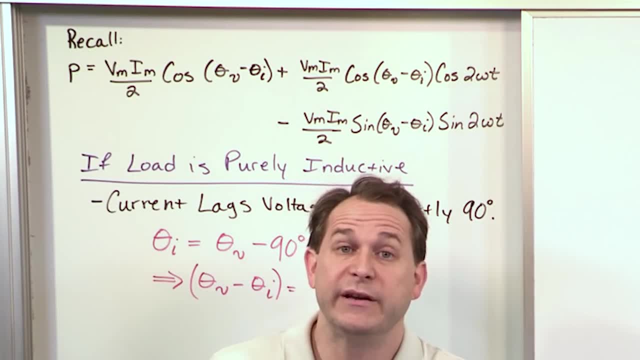 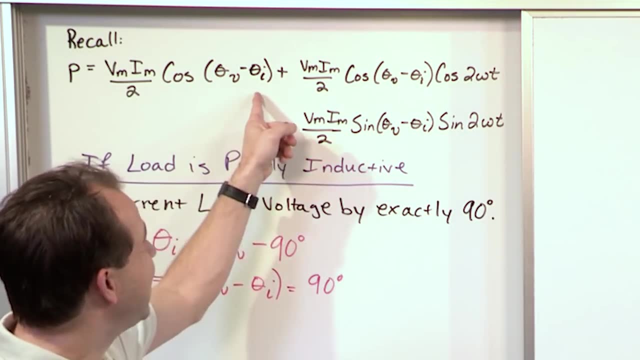 to drastically simplify this equation and make it something that we can study when the load is inductive right- Remember back to the last section, when the load was resistive, theta V minus theta I was zero, because the phase difference between current voltage 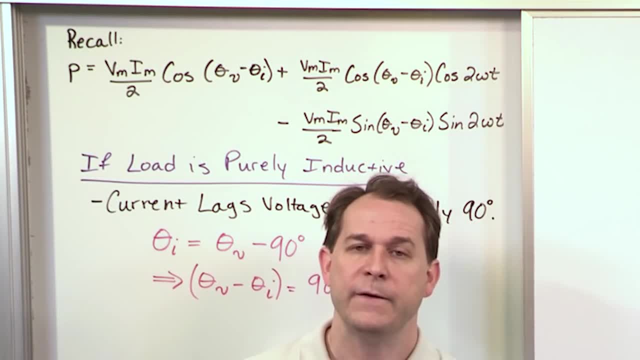 there is no phase difference between them. They're in lockstep with one another. When we say these guys are shifted by 90 degrees, we mean the sinusoids are shifted in 90 degrees along their horizontal axis, like that. So we'll actually plug this number in and study. 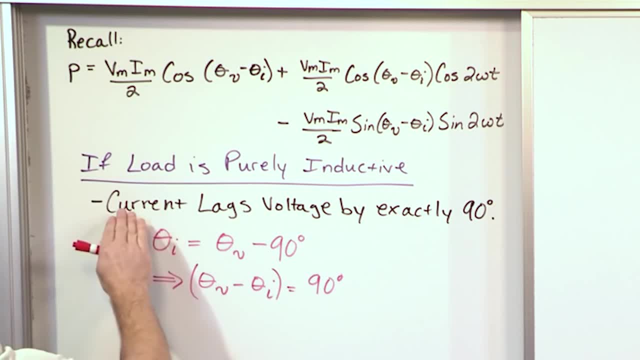 it for a second, But I want to talk for just a minute about this statement one more time. Current lags voltage by 90 degrees in an inductor, because I guarantee you will forget it at some point in the future And I want to tell you if you forget on a test, if it's leading or lagging. 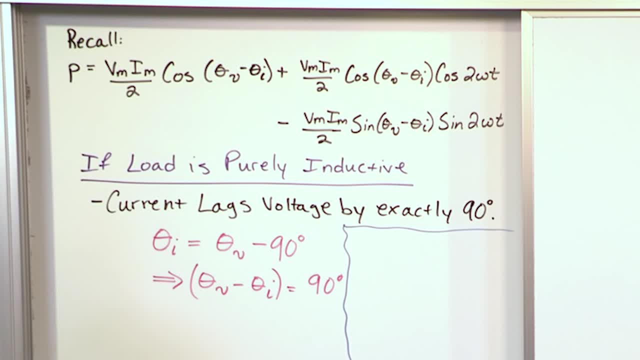 how do you figure it out for yourself? What it comes from is, if you remember back when we studied inductors, the voltage across an inductor is L, the inductance times di dt, So this is the rate of change. 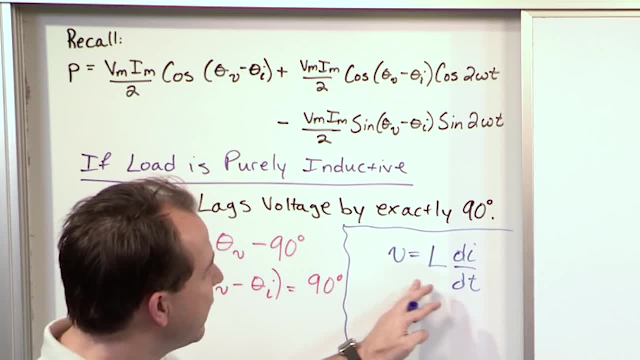 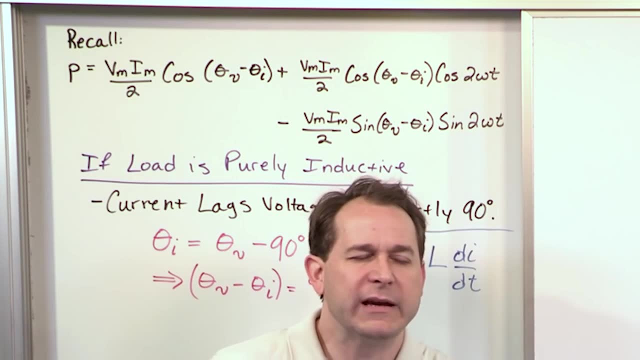 It's the derivative of the current flowing through that inductor. So you see, these are very interestingly related. The voltage is not related to the current. It doesn't matter the magnitude of the current. The current can be a milliamp or a microamp or a nanoamp. 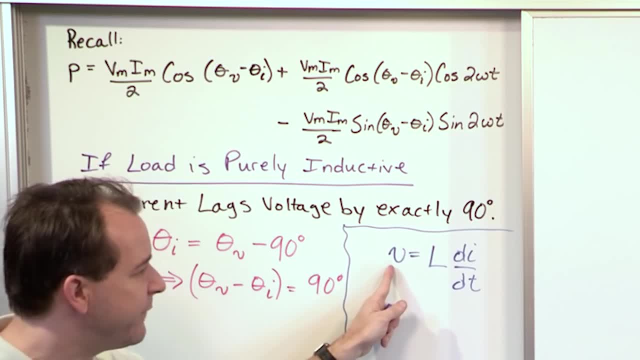 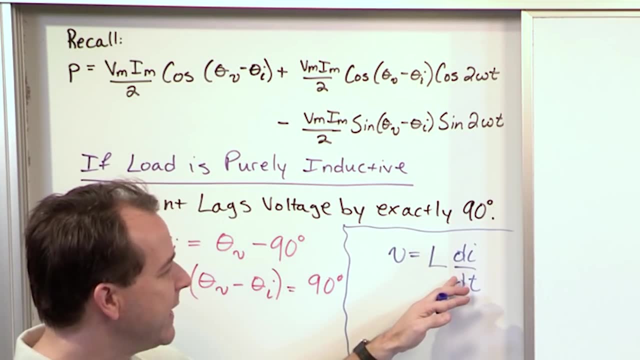 But if it's changing really really really fast, then you can have a very, very large voltage across that inductor. So even if you have microamps but it's rapidly changing super, super fast, then this di dt can be really really big, even if the current is. 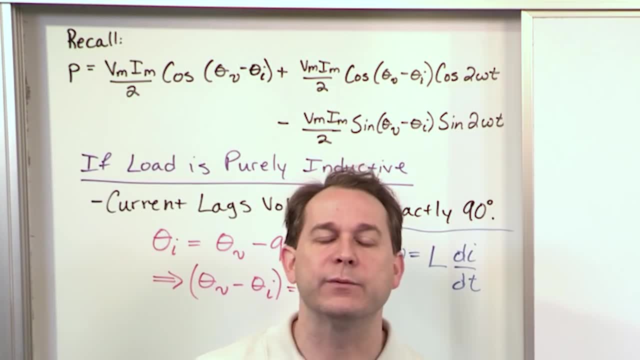 small. So you see, in an inductor the voltage is related not to the current, It's related to how fast the current is changing. And that is why these guys are shifted out of phase by 90 degrees, Because if you go and draw it here, let's go and actually draw the current. 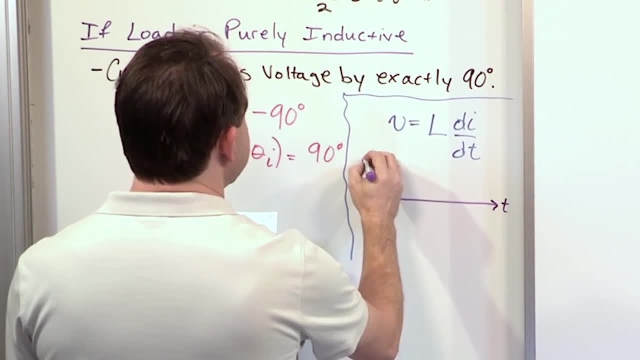 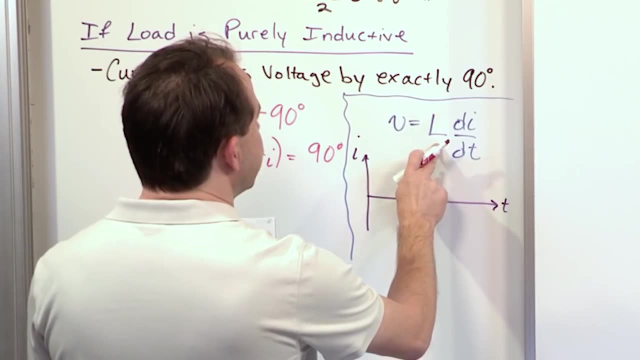 So this guy is going to be time And this guy is going to be the current through our inductor. So let's just say, for the sake of argument, that we're going to start out with a cosine. Let's just say we have a cosine because these are all cosine functions And 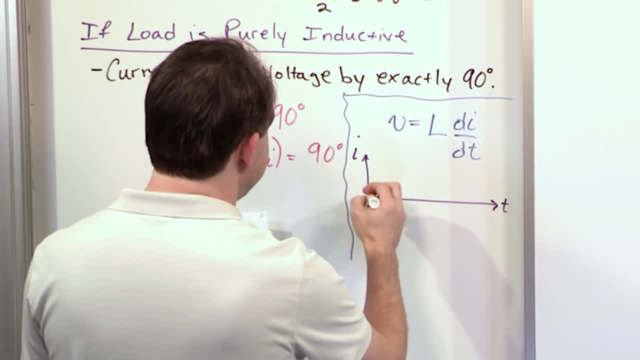 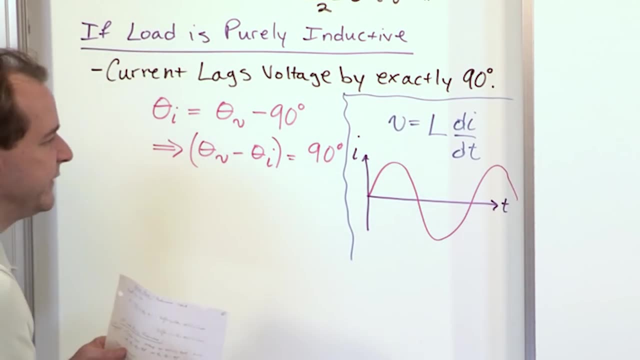 we're going to plot the current. So here is a. well, let's say it's a sine, Let's go like this, Start like this, like this, and so on. So let's just say, for example, that this is the current flowing through the inductor At time 0, it starts up like this and it 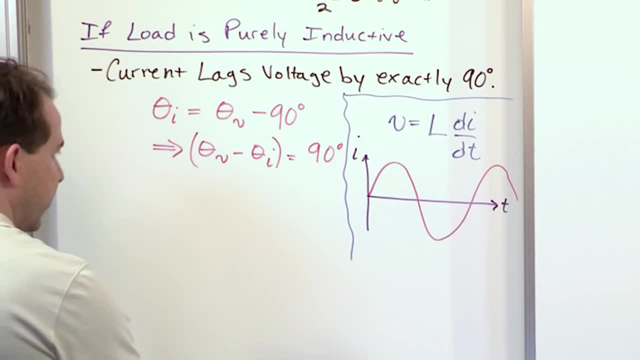 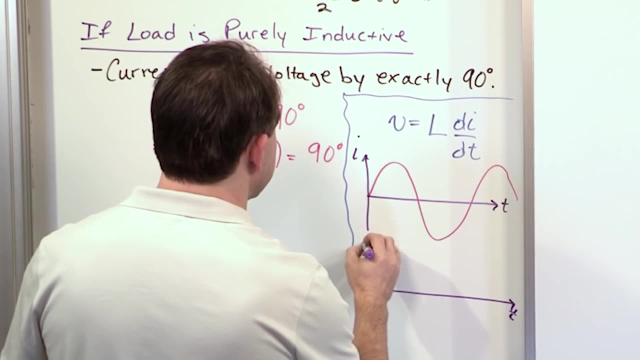 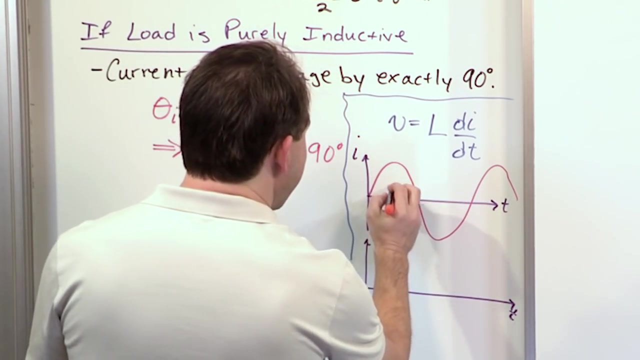 goes down and it goes up and so on. What is the voltage going to look like across that inductor? And this will be the voltage. What's it going to look like? Well, we need to draw some lines to help us draw some things here At the maximum. here I'm going to draw a little. 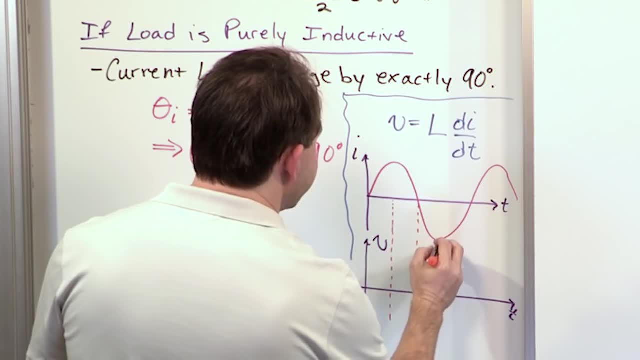 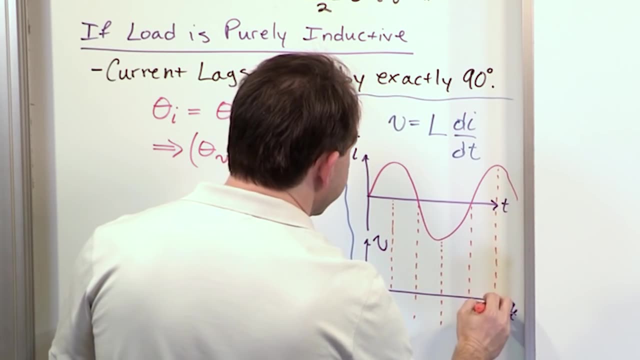 line here Where it crosses 0,. I'm going to draw a little line here At the negative maximum, we'll say it's right there, And then here at 0, we'll say it's right here And we can draw one more if you want at that maximum right here. So what we're basically saying. 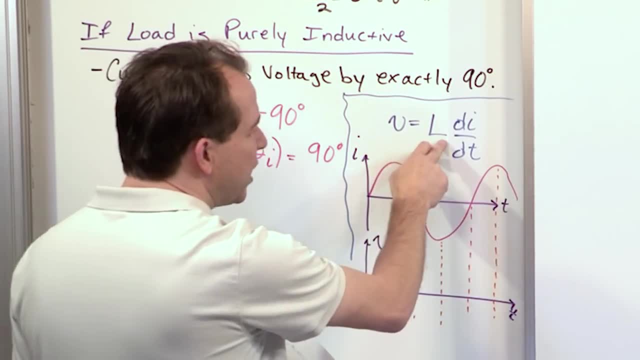 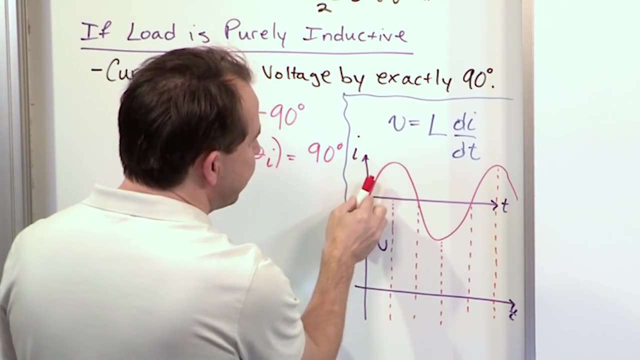 is that the voltage here that we're plotting is some constant times di dt, Now right here, as it's crossing through 0, this guy has the maximum slope it's going to have. The derivative is a maximum right here. So the voltage is going to start at a maximum value And then 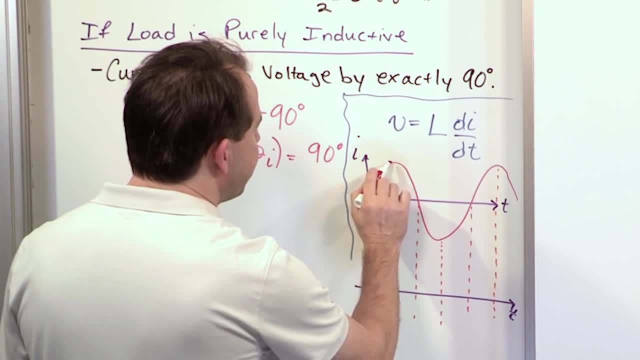 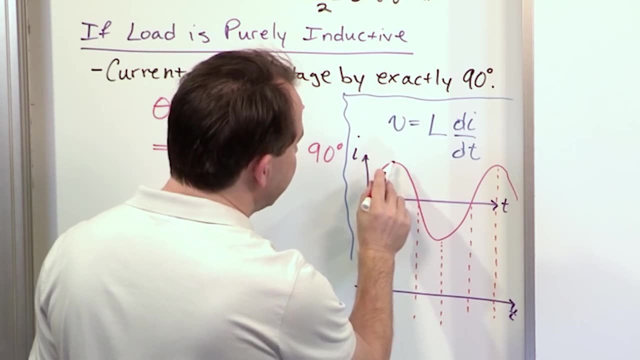 what's going to happen is: it's going to go. this guy's going up, up, up, up up. Eventually it gets to the plateau. here at the top, The derivative is 0, because the function is not changing anymore here. So what happens? it's going to go like this. This guy's going to 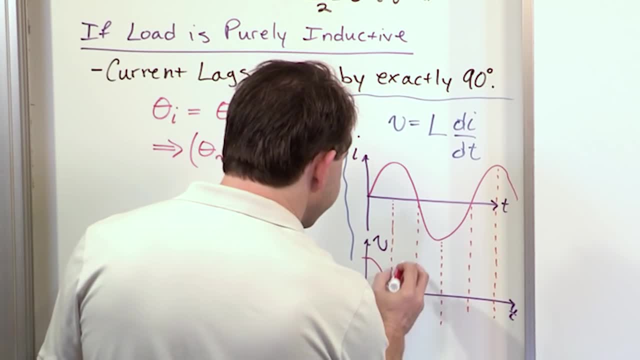 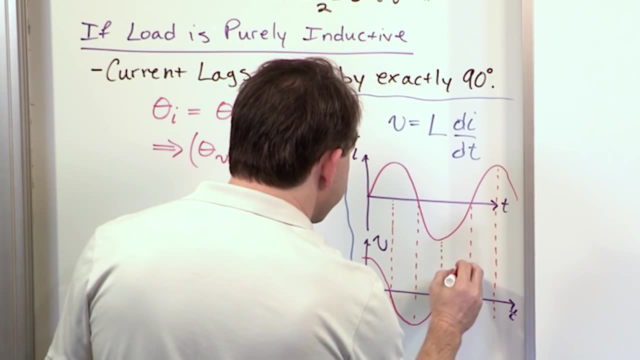 start to bend down and it's going to go through here And I'll just continue drawing it for you here. It goes down below to a negative maximum here, up through here, and then it goes up through a negative And then there's a maximum here And then it goes down like: 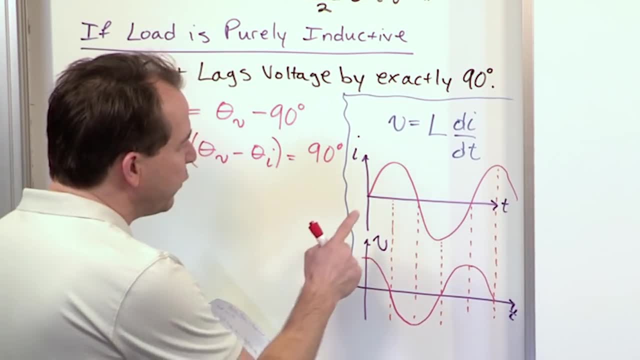 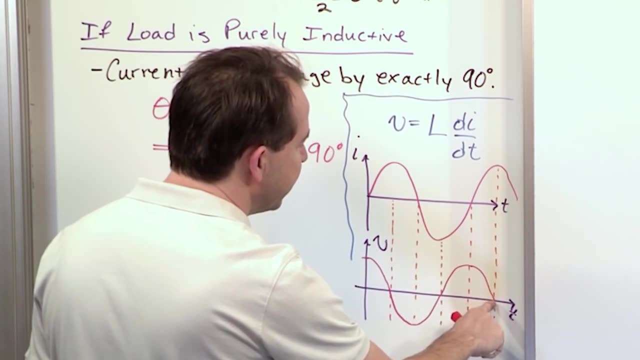 this. So this is what it's going to look like. Make sure you understand that. so you see, everywhere there is a peak, the derivative should be 0.. Here's a peak, and the derivative should be 0.. Here is a peak. the derivative should be 0.. Here the derivative is a maximum. 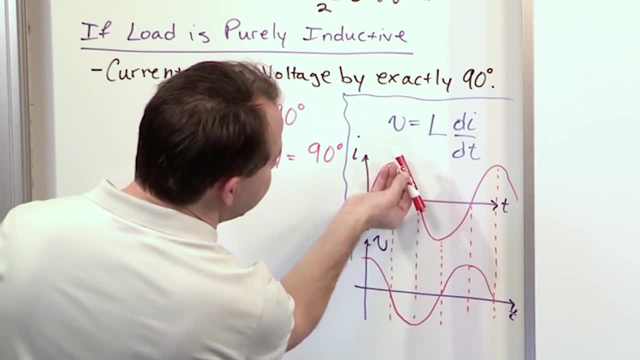 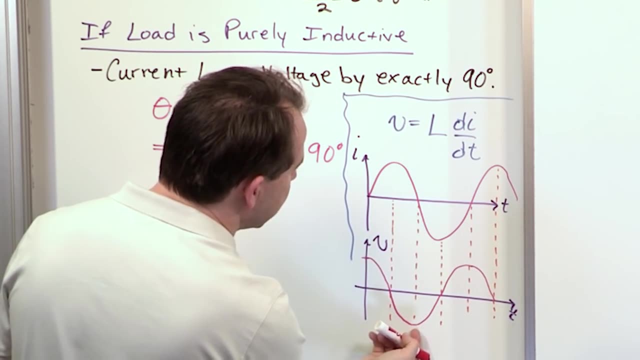 positive number because it's sloping this way And as we go down this way the derivative also is a maximum. but it slanted the other direction, in the negative slope direction, So we should have a negative maximum here. Here the derivative is sloping back positive. 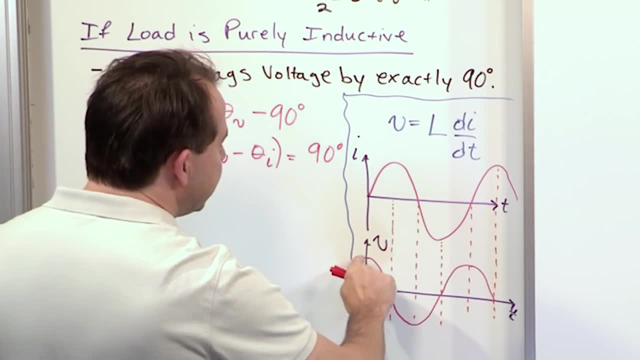 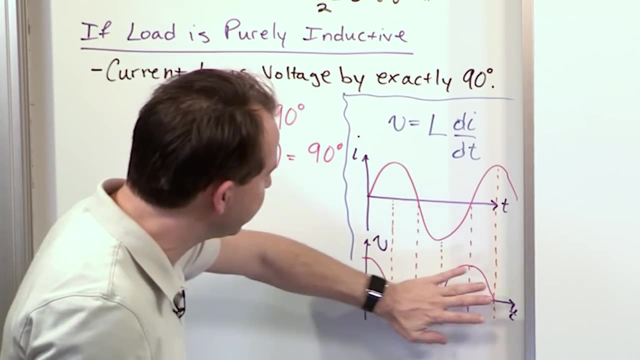 here. So you see, what's happening is everywhere in between the thing is changing and it's just kind of crossing through these points. So this is nothing new. This is basically a sine, and here's the derivative. We know the derivative of sine is cosine. That's what I've drawn here. All right, But what I want you to, 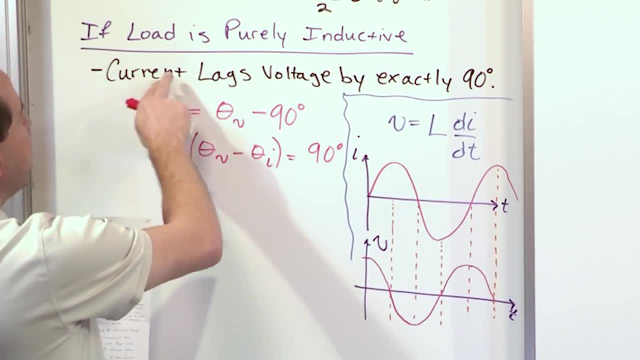 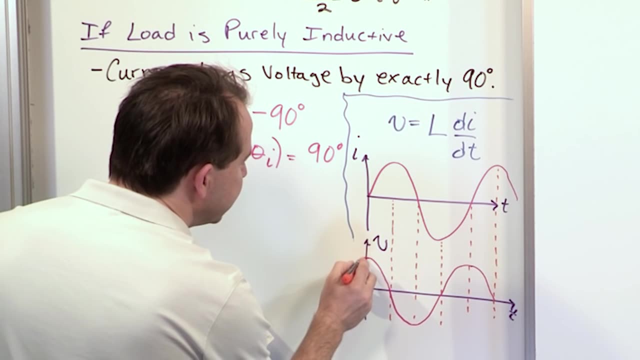 notice is that what we said here current lags voltage by exactly 90 degrees. Make sure you understand that. It's a little easier to understand it if I actually kind of do a dotted line in the negative time direction, like this Right Current. 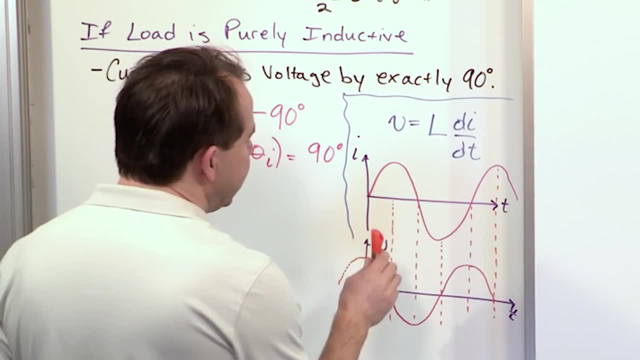 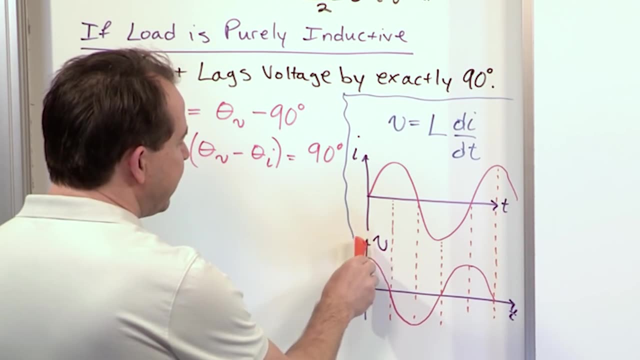 lags voltage. What that means is that any point in time- right, Let's pick. right here, This is the voltage, right here, We're saying that right at this point. here's what the voltage is looking like. The current is going to lag that guy by. 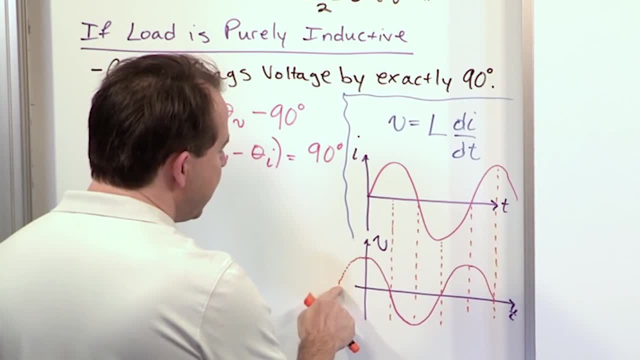 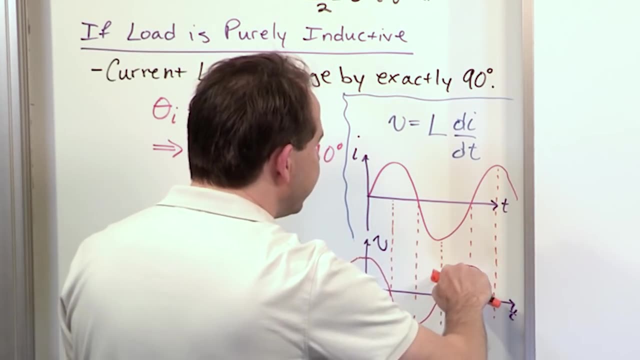 90 degrees. So if I take this guy and go 90 degrees to the left, this is exactly what my current is doing at that point in time And that's what's basically happening. If you pick any point along this voltage curve, let's say this point: 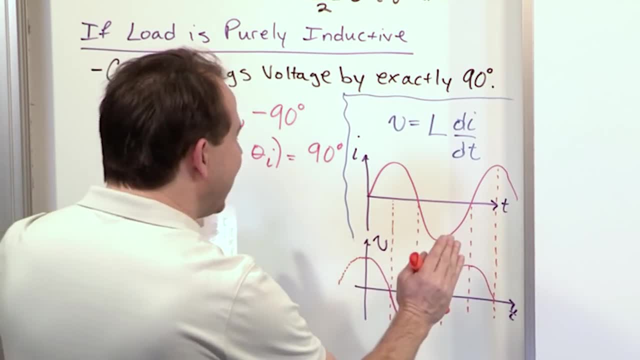 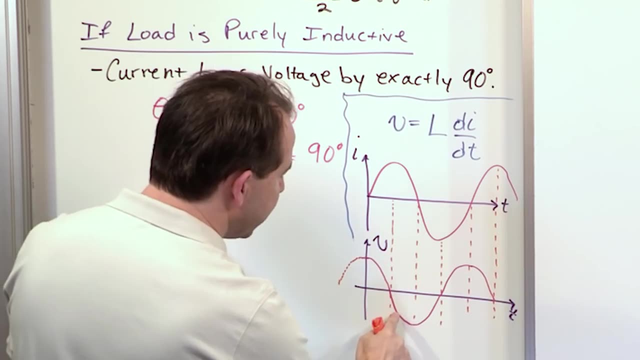 right here, this maximum right. We say the current lags the voltage. So basically the voltage hits the peak first, and then a little bit later the current hits the peak. The voltage here hits a trough here and a little bit later the current hits the trough. So you, 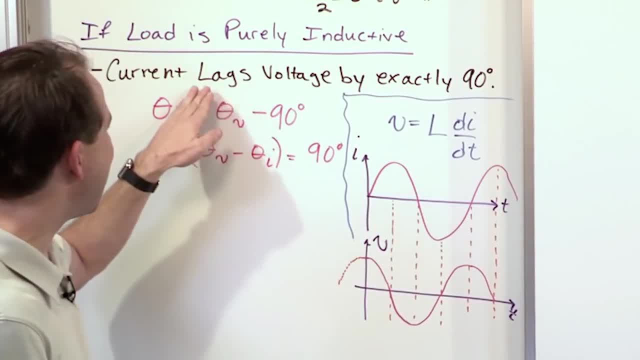 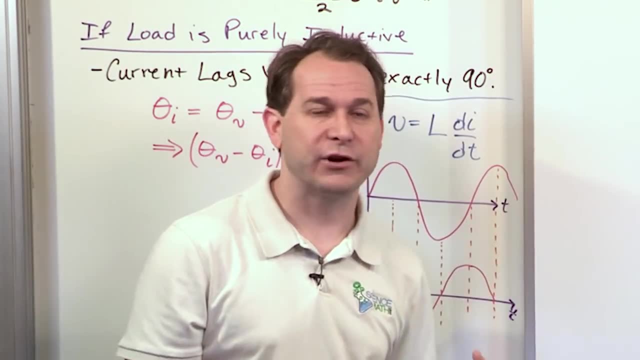 see, the current is lagging the voltage. right, The current is lagging the voltage by exactly 90 degrees because, as the voltage gets to wherever it's going, 90 degrees later. okay, then you have the current doing the same thing, So it's a. 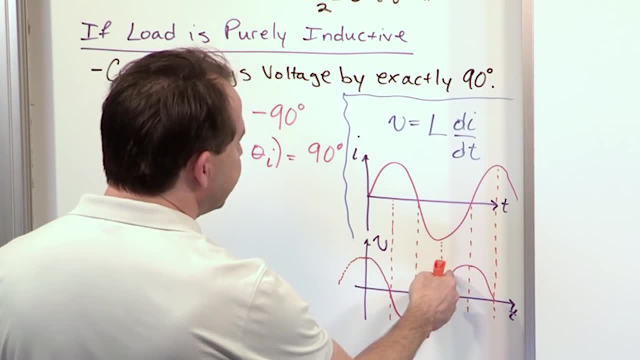 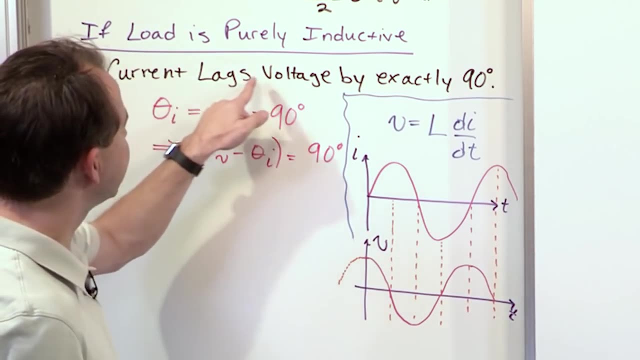 little bit of a delay there. You can look at it a couple of different ways. If you take this guy, shift it to the left 90 degrees, that's what's happening. That's your on your curve at that point. So if you forget that, the current is 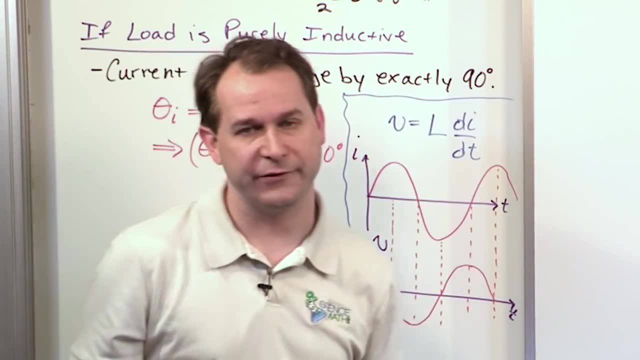 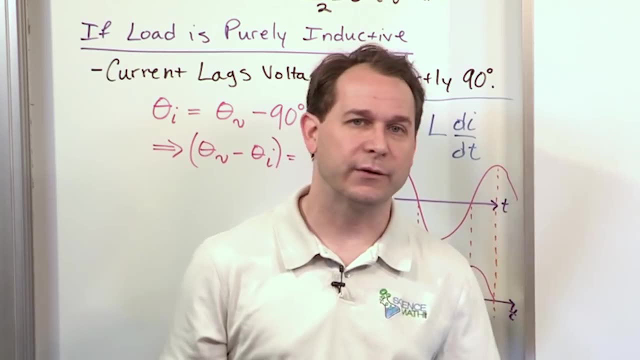 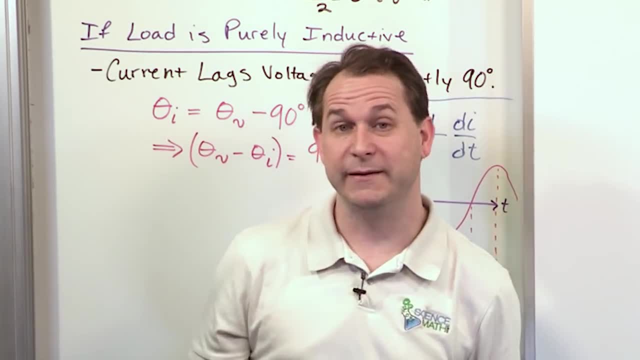 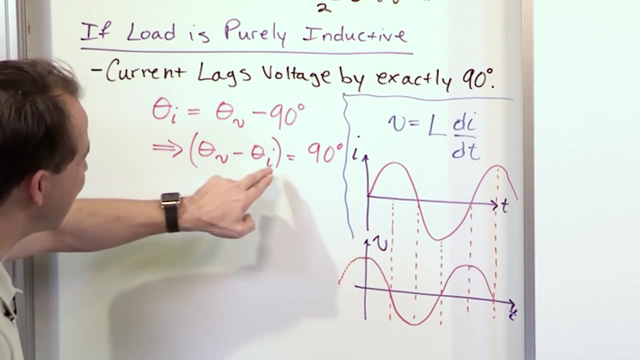 we get to capacitors, it'll be. I don't want to confuse you now, but it'll be a little bit different. So this was an aside. The point of this was to show you that theta V minus theta I is exactly 90 degrees. 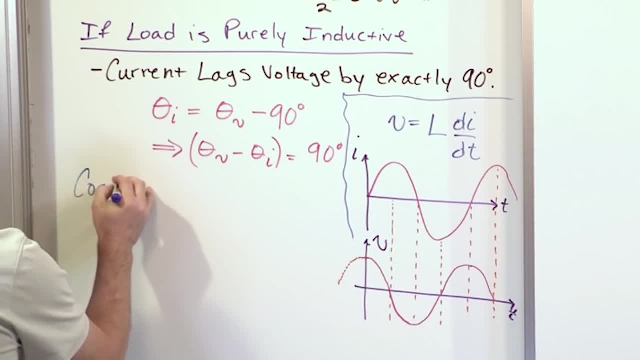 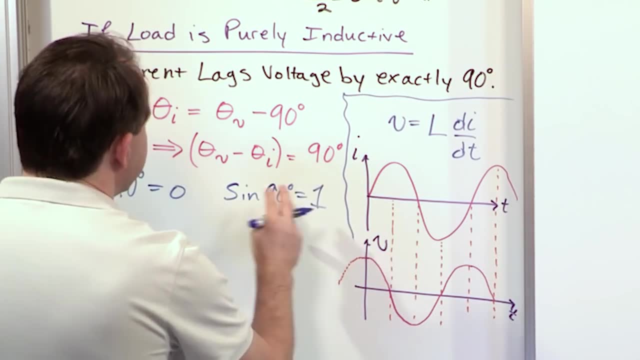 And you should all remember that the cosine of 90 degrees is going to be equal to zero and the sine of 90 degrees is going to equal one. So let's take this information and we're going to go over to the right-hand side of the board and 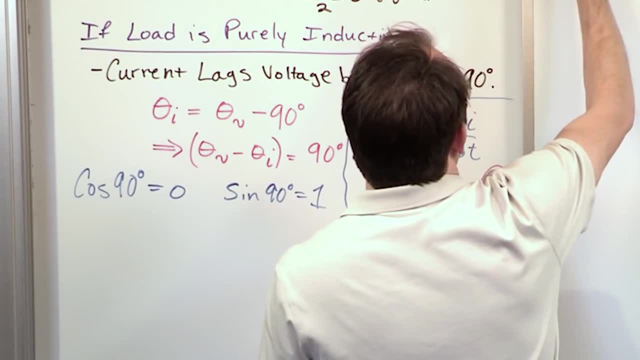 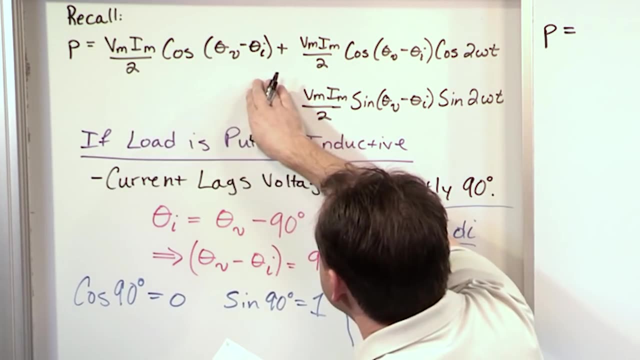 write down what the instantaneous power looks like. now that we know that it's an inductive load, What we have, this first term is going to actually disappear, because it'll be cosine of 90 degrees, which is zero. So this disappears, right. 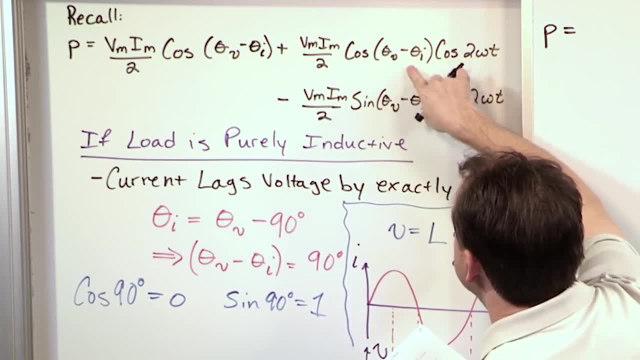 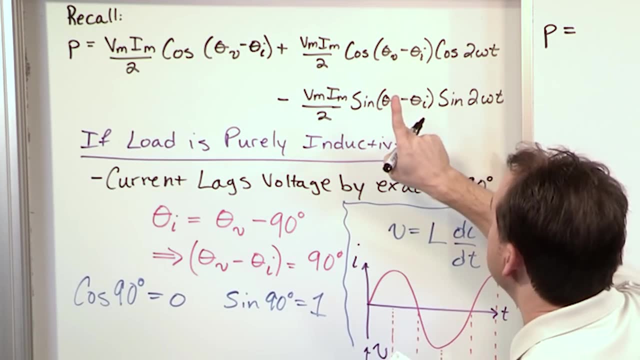 Here's a cosine of 90 degrees, So this disappears too. So the only term that we have is this term, but notice, we have sine of 90 degrees. Sine of 90 degrees is one. So the only thing here in this instantaneous power is the negative. 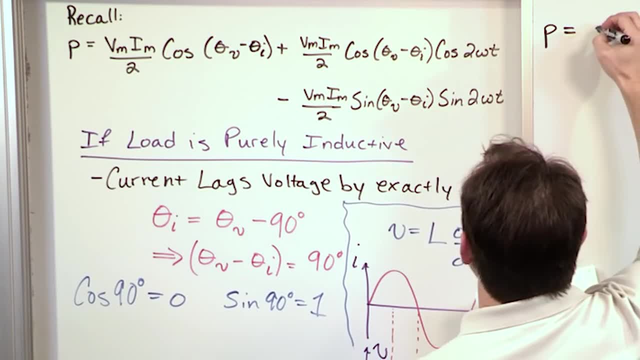 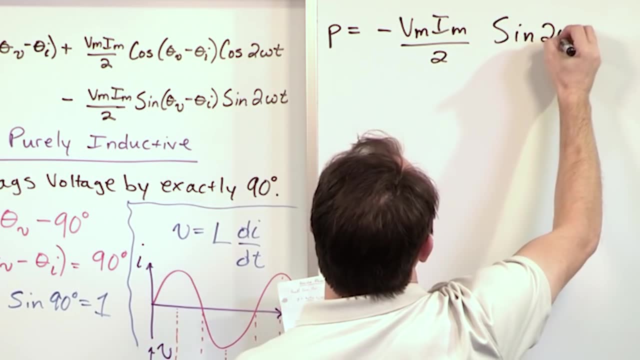 these coefficients here and then this guy at the end. So what you have is negative Vm. I m over 2 times the sine of 2 times omega t. So this is- I'm going to switch colors. this is really important. 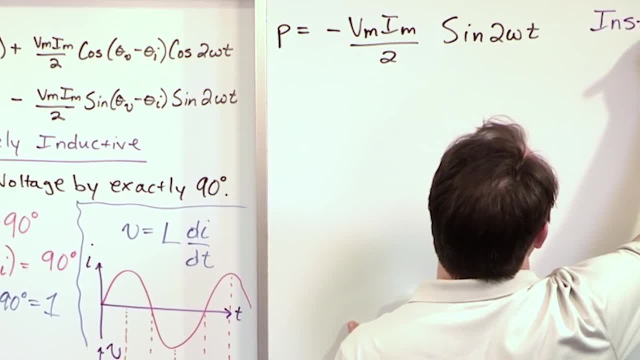 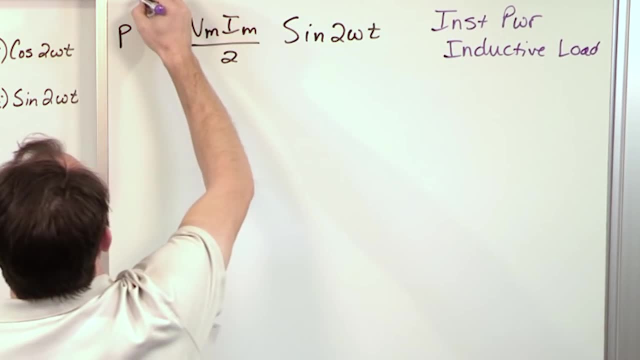 This is the instantaneous power when we have an inductive load. All right, so I'm going to kind of circle this Now. I am going to kind of caution you, here I'm giving you a lot of theory, here You're not going to use these instantaneous. 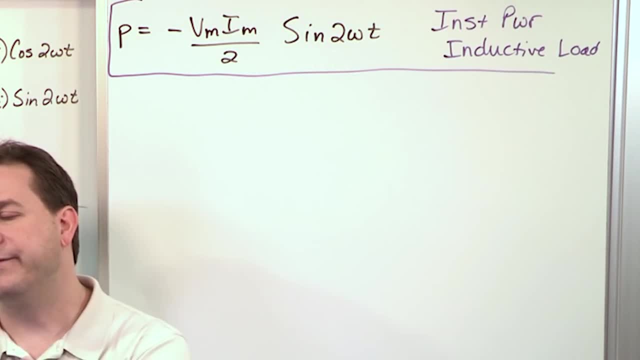 equations much when we're doing real circuit analysis, We're going to use phasor techniques and other things. but I'm trying to really show you where all this stuff comes from, because you will probably have a few questions on it. and, more than anything else, the books. a lot of them are really hard to follow. 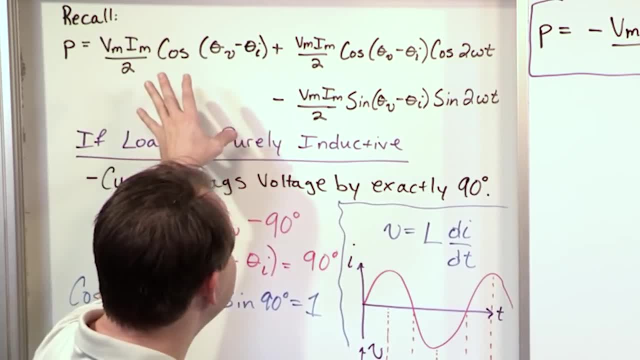 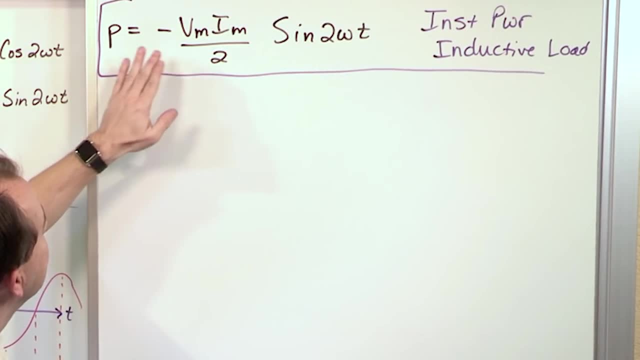 And what's happening with this math? here? All we're doing is taking this instantaneous equation. We know what the phase difference is for an inductive load. Most of these terms drop away, and here is what it really looks like for an instantaneous power in an inductor, when you have purely inductive load. Now the 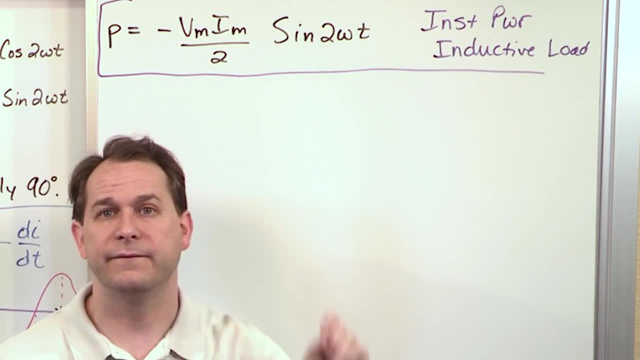 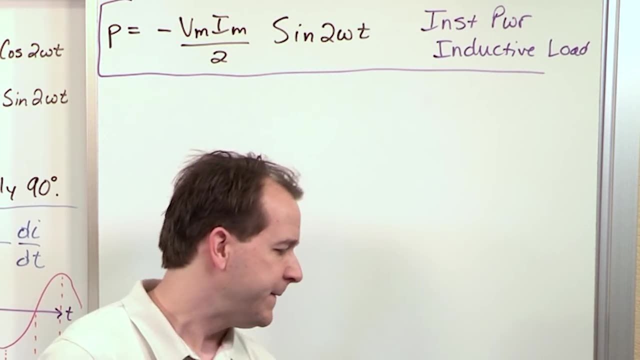 rest of my lecture is just going to be some comments about this very simplified equation. because now we have just inductive load, everything drops away. So I'm not going to write too many things down, but I'm going to make sure you understand everything. 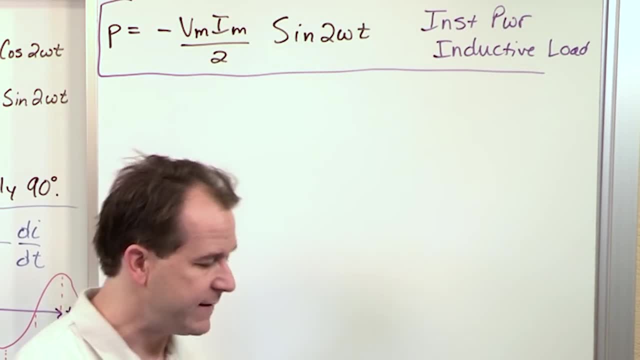 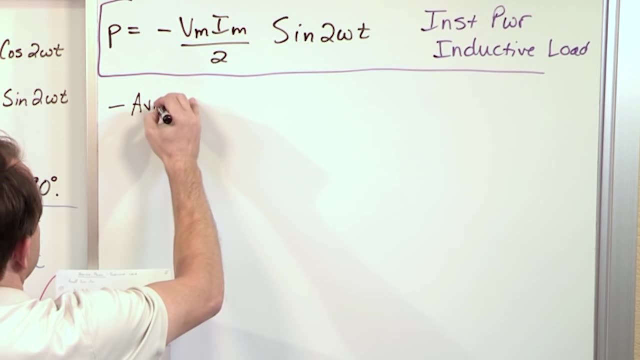 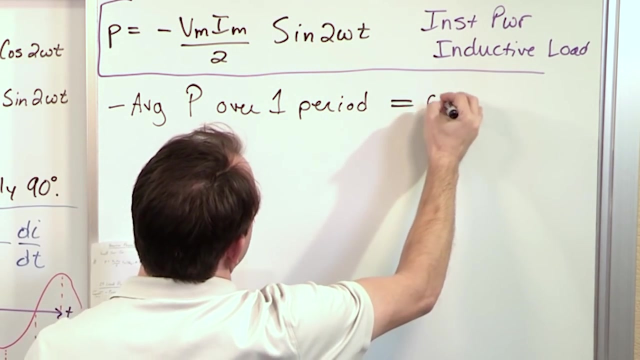 All right. First thing is, the most important thing is the average over one period. Actually, I'm going to write this one down, So I'm going to put the average power over one period is zero. Make sure that sinks into you. Okay, Remember we. 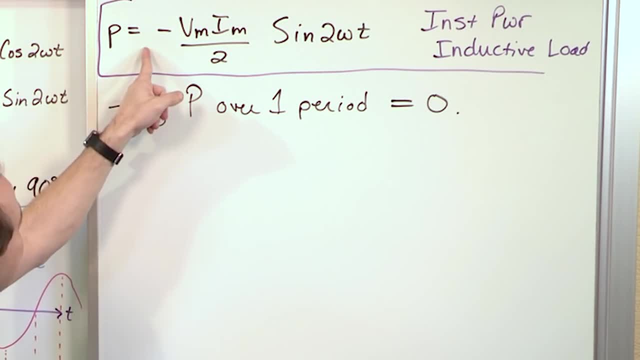 talked about. how do you calculate the average power over a period? Well, you integrate the instantaneous power over DT over one period and then you divide by T. We talked about that just in the last section. So if you were going to figure out what the average power was here, you would take this guy and you would 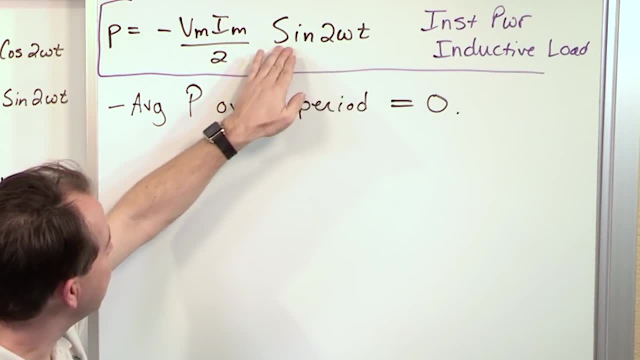 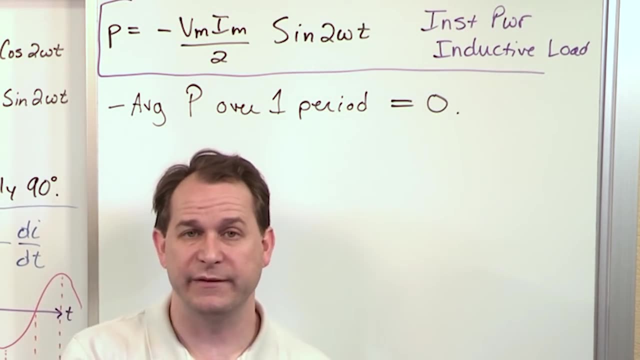 integrate it, But notice that it's just a sine right. It's got two omega T, but you're integrating over one whole period, So you've got a doubling of the frequency. So you have this in a similar way for the resistor, The frequency is 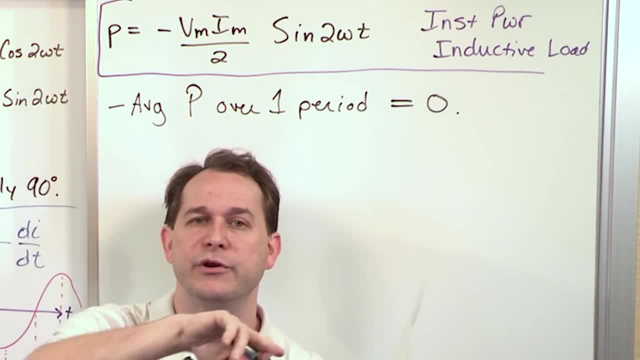 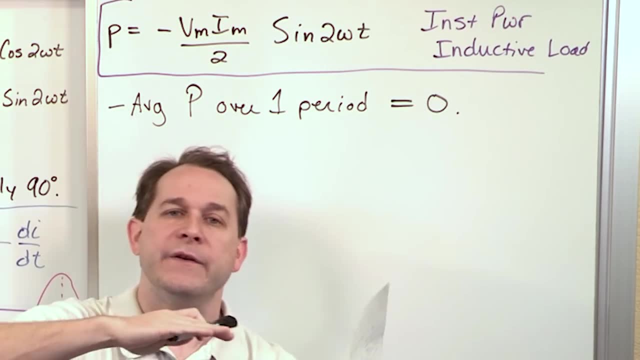 doubled right, But you're still integrating over a complete period. So you're going to catch that sinusoid exactly where it starts if you start anywhere and integrate over one entire period. So since it's a sinusoid, it's going to stop at any point of time. as much as possible, What's evenly. 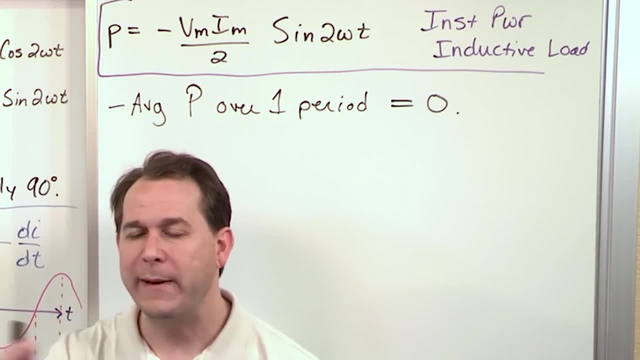 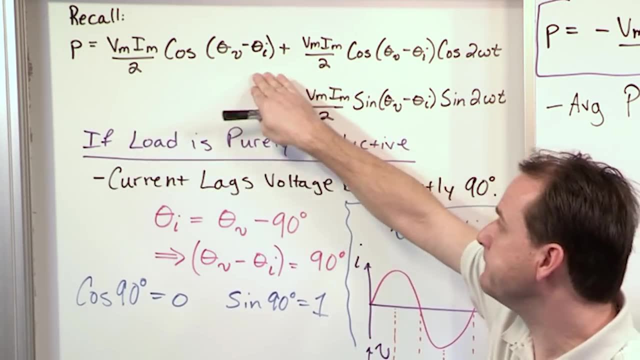 distributed Right, All right. filed All the way above zero and start back at zero. same thing over two periods. Right, The same thing over two periods. Same thing over two periods. So what can you do? What can you do Our calculators talk about its shape, right. So some parts of the carrier are in two link cells and so some parts of the carrier are inside of that R trend. You say this is sort of a power division. were hardest to understand because you're going to try to figure out how much. power you can get, but it doesn't exactly give you the value you value. you get tiny Data, Alright, so here's what the average power is delivered to a resistor. Remember, go back to the last section. we talked about the average power. It was a non-zero. 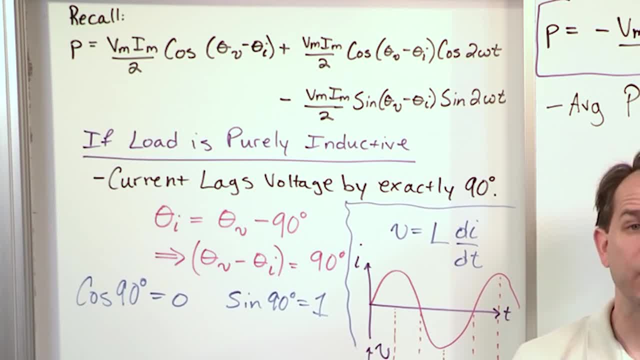 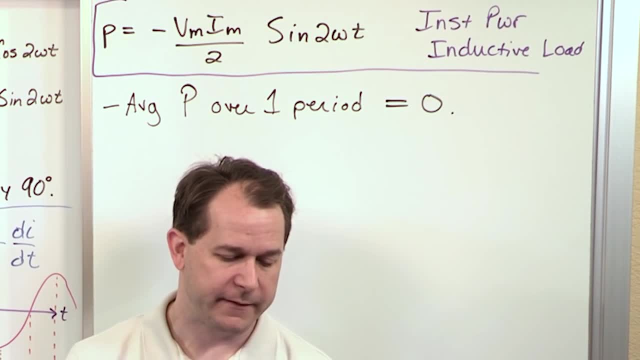 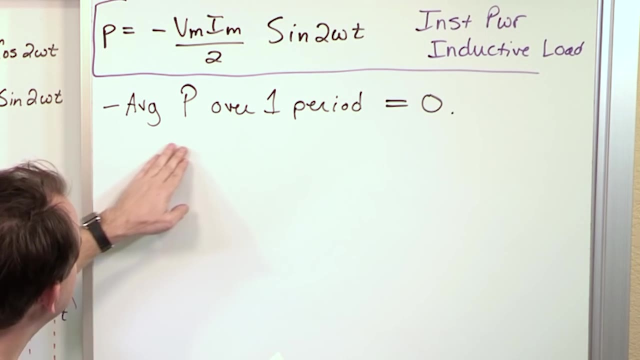 resistor, But in an inductor the average power is zero, right? If you look forever and ever and ever, the average power is zero. okay, for an inductive load. So that also another way to say this- is that there's no transfer of energy from electrical to non-electrical. 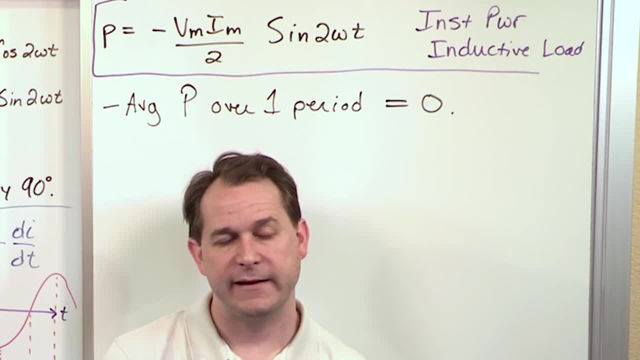 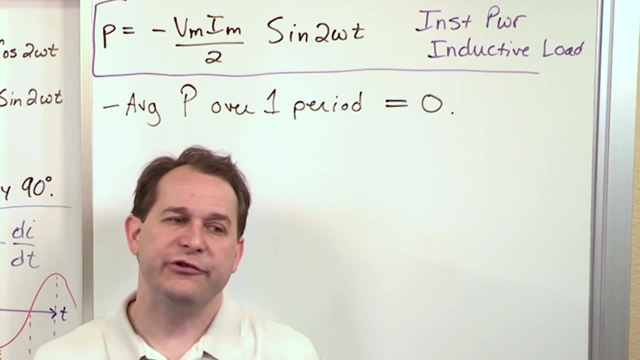 form in an inductor. So in a resistor we say that the power is delivered to the resistor and it re-radiates it out as heat that's lost to the environment. In an inductor, the energy that you deliver to the inductor during half the time gets stored in the magnetic field. 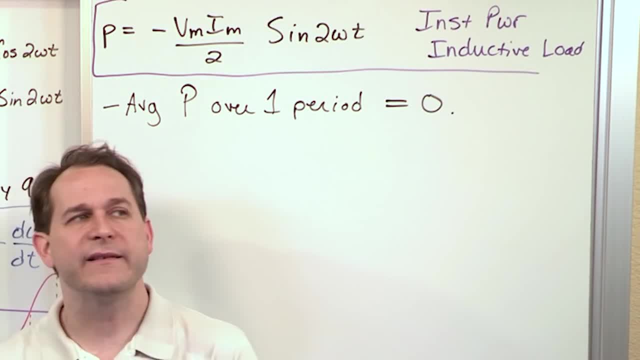 in the inductor And then the other half the time the energy is kind of pulled out, but it doesn't ever get dissipated to the environment, It's not lost to heat, It goes into the magnetic field and it comes out and kind of is transferred back to the circuit. So it's a sloshing effect. 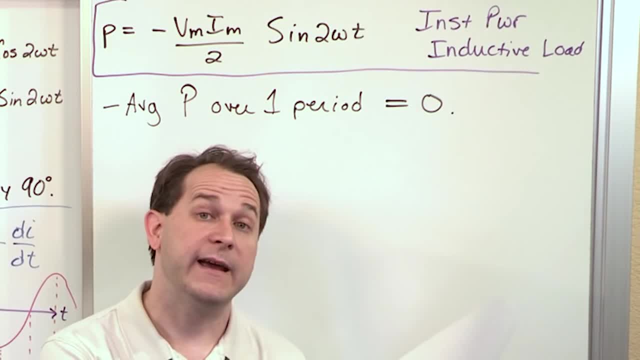 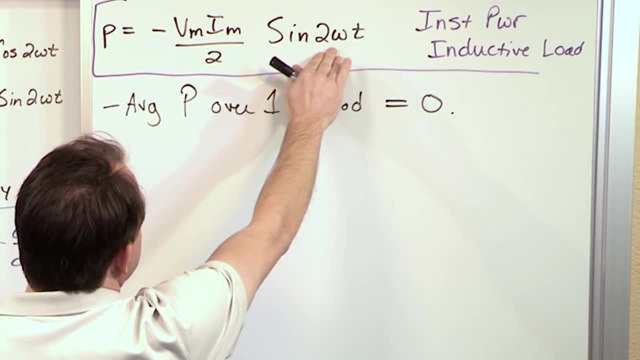 back and forth: delivered and then taken from, delivered and then taken from. That'll be a little bit more clear in the other here in a second. The instantaneous power is twice the frequency of the original frequencies that we're talking about. So we that's kind of similar to the way it looked for for the resistor, And I already 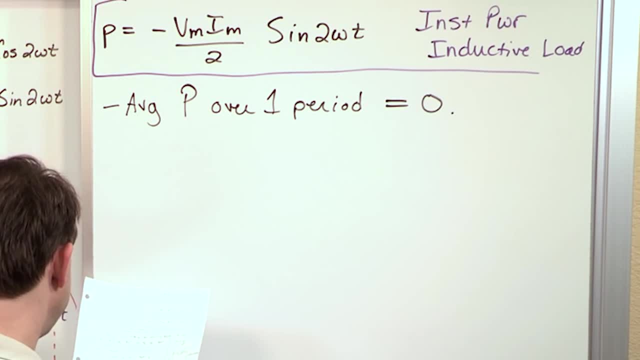 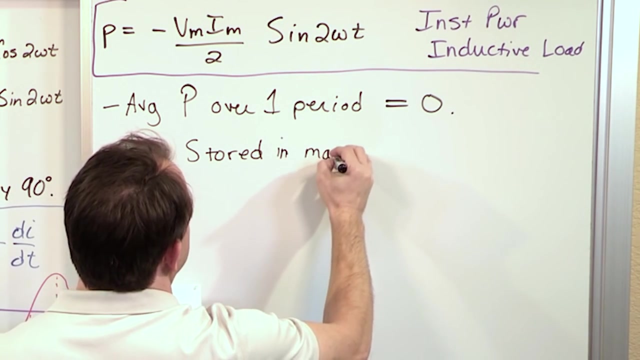 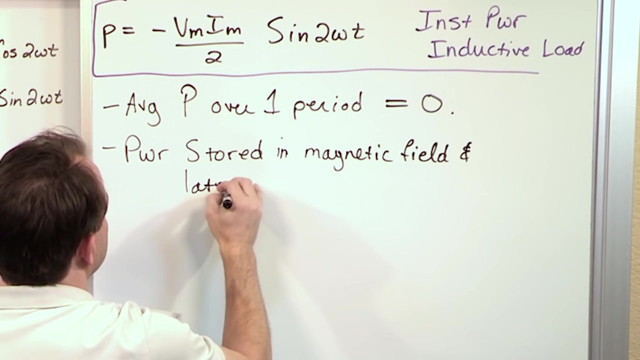 said this power is stored in the magnetic field and then later extracted. So I want to talk about that. Power is stored- and I'm using these terms loosely, Um, you know, it's really- energy is stored in the magnetic field, in the magnetic field, and later extracted. 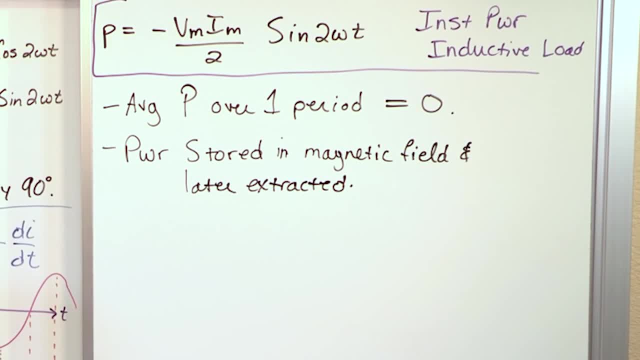 All right. Now, what do I mean by that? Notice that this instantaneous power is a is basically a sine function. It's got a doubling of the frequency. That means and we have a negative sign there. but that means sometimes this instantaneous power is going to be positive. 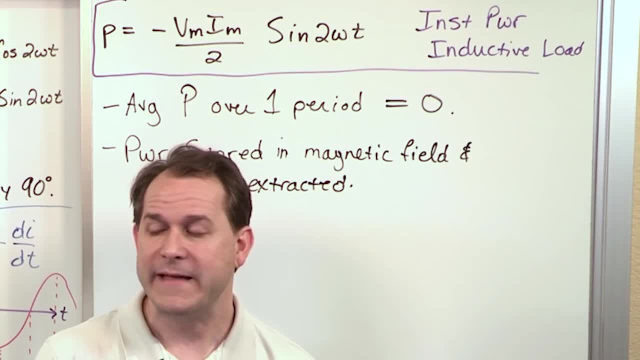 and sometimes the instantaneous power is actually going to be negative. That did not happen for a resistor- If you remember, that thing was oscillating above the horizontal axis- It was never negative. But for an inductor, everything else drops out. This is what we're. 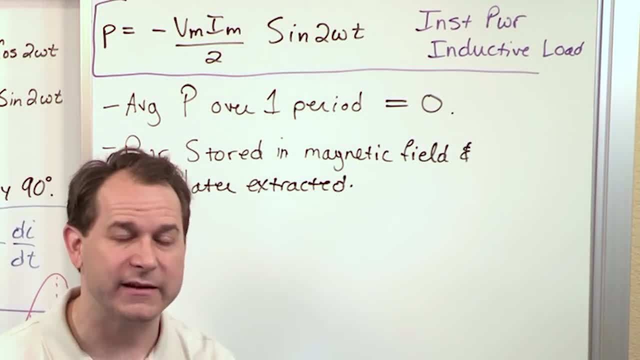 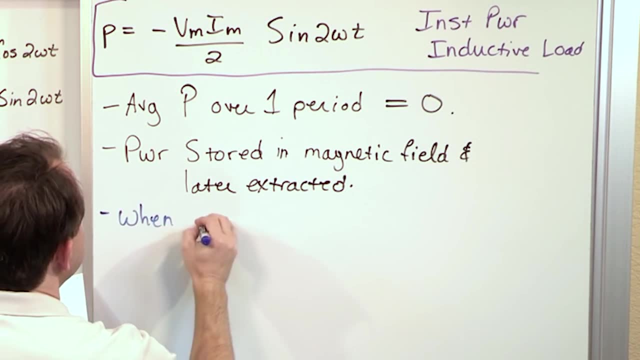 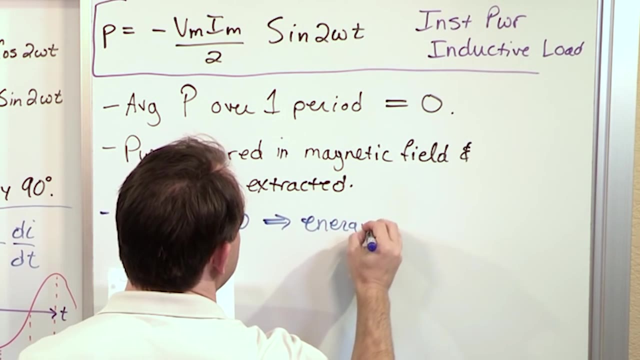 left with. Ladies and gentlemen, half the time instantaneous power is positive, half the time it's negative. What does that physically mean? What that physically means is when the instantaneous power is positive, when it's greater than zero, that means energy is stored um in. 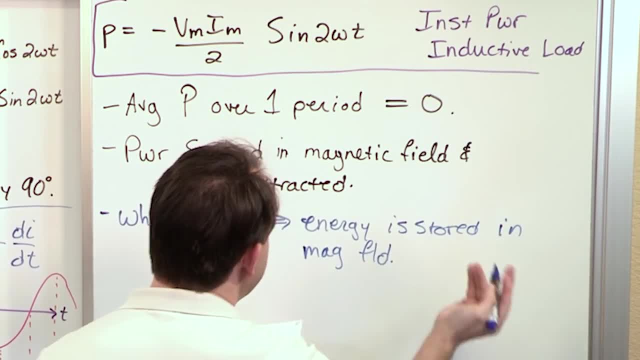 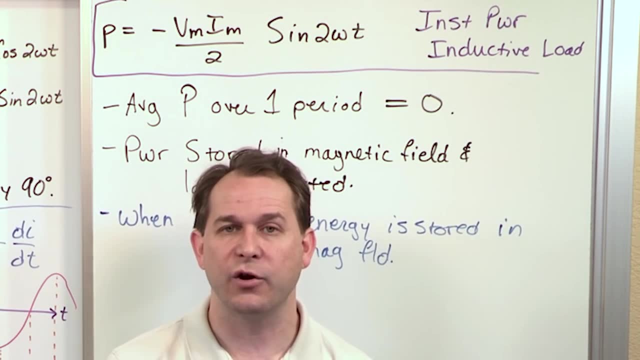 the magnetic field. And what magnetic field are we talking about? Don't forget, in an inductor is a coil of wire. The reason it's coiled like that is to concentrate the magnetic flux inside of that coil, So the energies actually stored in this invisible thing we call the magnetic field. and it's, it's a real thing. 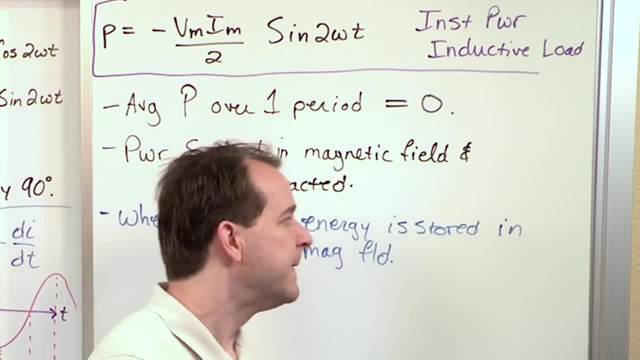 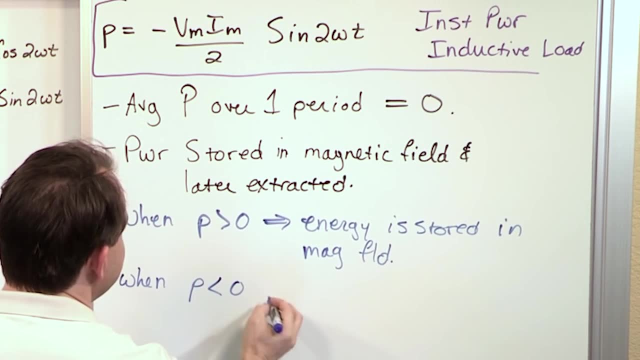 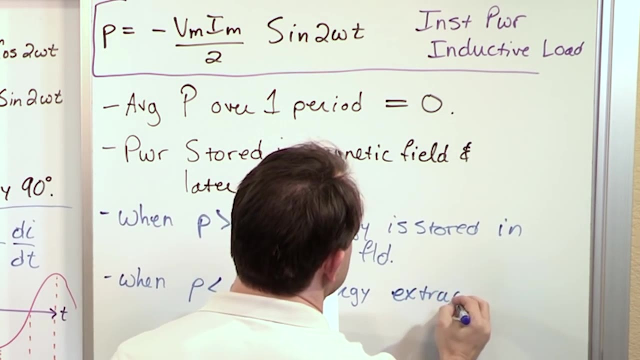 It's energy stored there that can do work later on down the line. When does it come out? is when, during part of the cycle, p that we calculate here is less than zero. So when it's negative, the energy is extracted from- uh, the, if I can remember correctly, from one of the inner circuits of the magnetic. 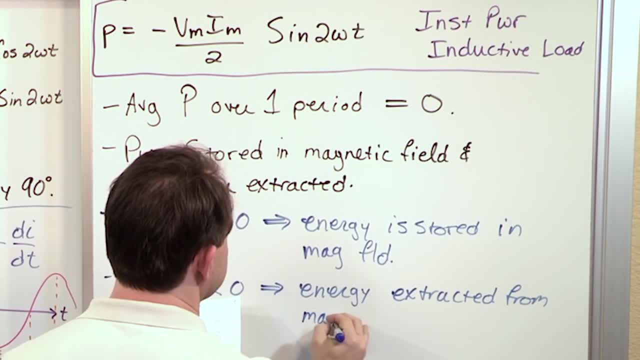 field, So from one power to another. uh, this is a magnetic flux that's stored in this invisible, the magnetic field, or from the inductor, however you wanna say it. That's really, really, really important. and this is kind of where I start to get. 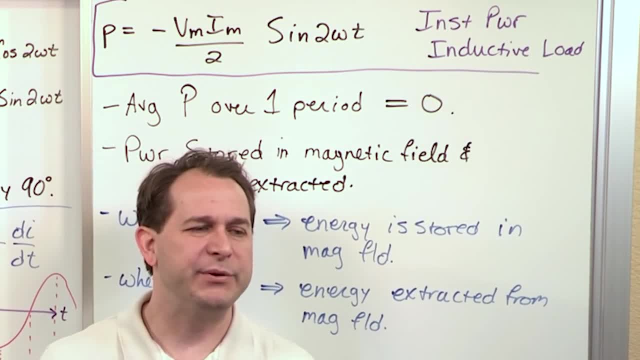 a little bit excited about teaching this kind of stuff. It's really a beauty in symmetry. what's going on here? You have this device. it's a coil of wire. If you stick a current through it, it concentrates a magnetic field inside the coil. 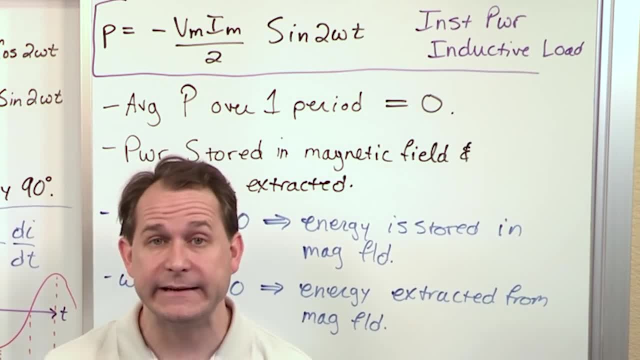 And magnetic fields. we can't touch them or taste them, or even see them, but we know that they can store energy. And then you say: well, how can something that's invisible store energy? right, How does that even work? 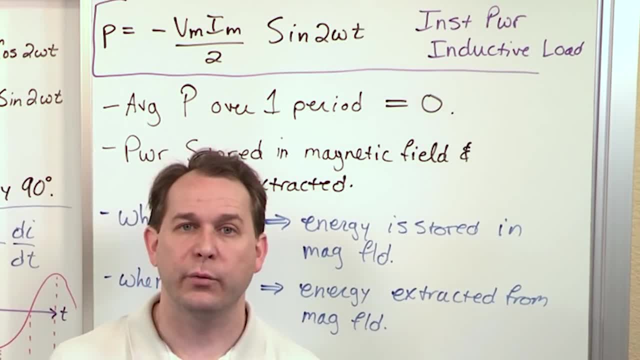 Well, what's happening is that all of these circuits we're talking about are sinusoidal. That means they're driven by sources that oscillate up and down And that means that for the inductive components, some of the time the power that you calculate- 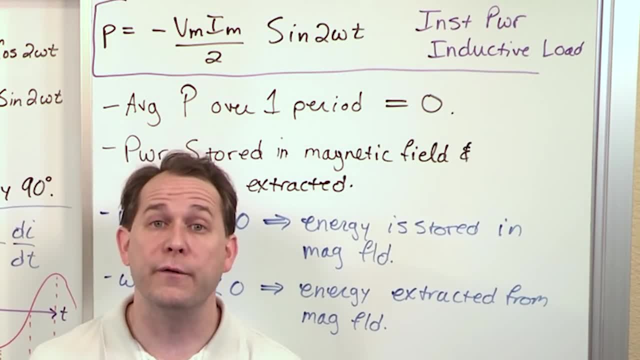 across the terminals of that inductor is gonna be a positive value. And we know from our sign convention of power: when you have a positive power that means energy's being delivered to that load, For resistive it just gets dissipated into space, it's heat. 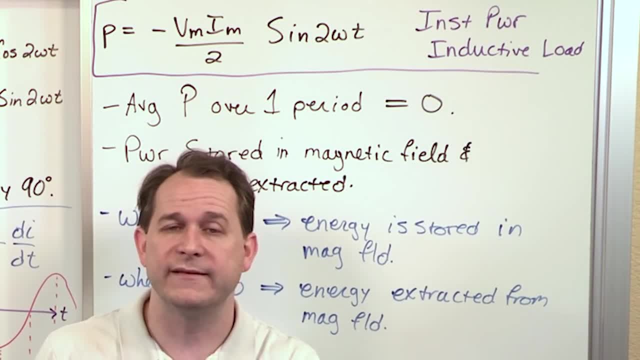 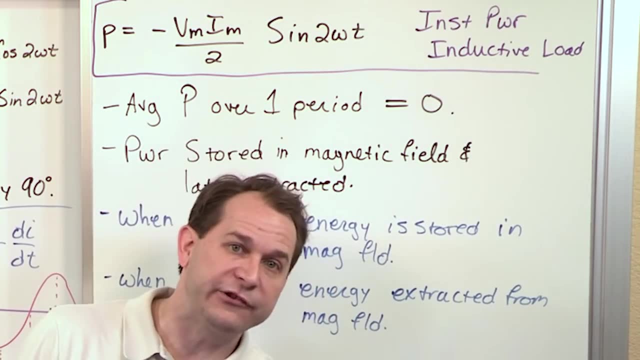 But when we're talking about that inductor, it doesn't get dissipated, it gets stored inside the magnetic flux, inside of the coil of wire that we have right, But then later on down the line the source swings the other direction. 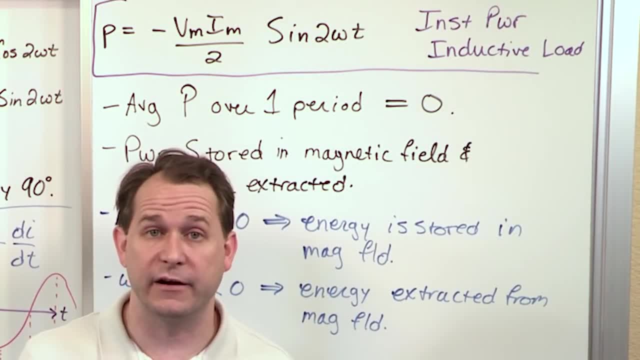 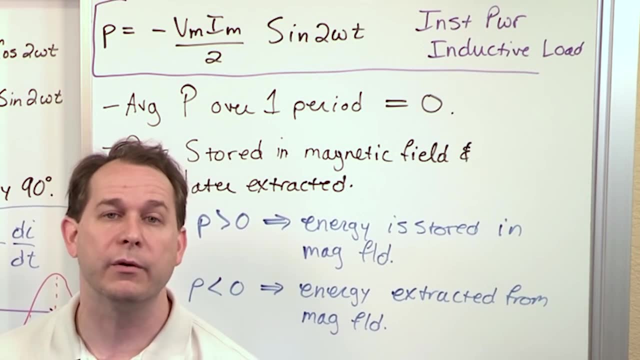 and things oscillate back the other way and then current starts to come out of that inductor And then some of that energy is extracted from the magnetic field, because then the magnetic field collapses down to zero again And, as it happens, that magnetic field 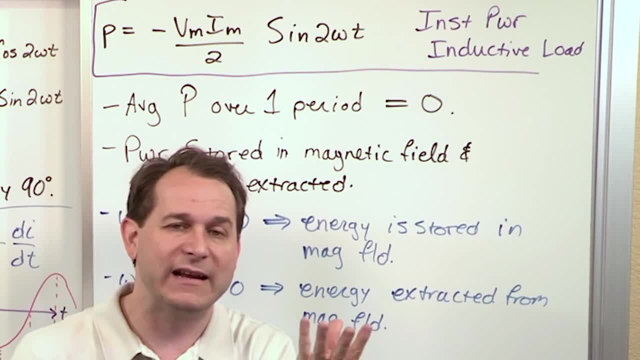 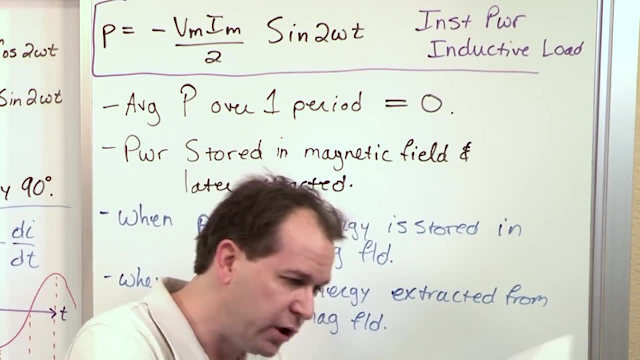 which is storing energy, is contributing to the current flowing out of that inductor as it collapses down. And that's a very real thing. I mean, if you put a lot of energy in a magnetic field and then you unplug it and you hook it up to something. 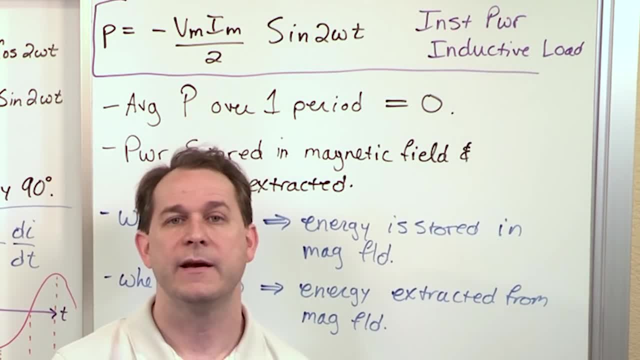 I mean you can see the current bleed out of that as the magnetic field collapses, And so that's real energy transfer. So it's kind of like a temporary battery. You can't. you know, it's not practical to like power a car. 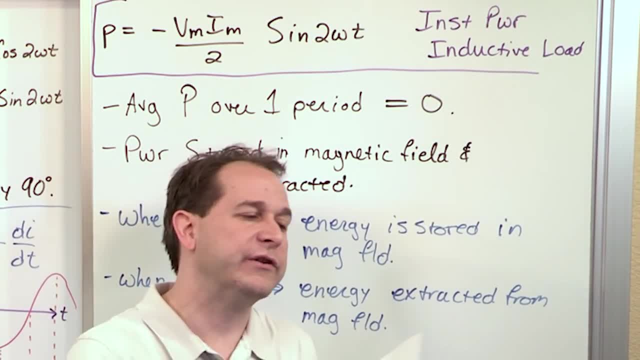 with inductors or anything like that, But as a temporary storage device you can store energy in an inductor when we're saying the power is positive part of the cycle here, and then we can extract it whenever this is negative. Remember: 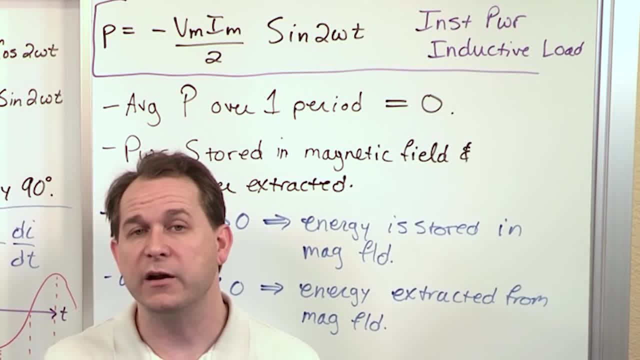 when we're talking about our circuit analysis. we've done all along, we've done power calculations And for the resistors you always find the power is positive. But for the sources, even back in DC analysis, you usually find, you always find- that the power 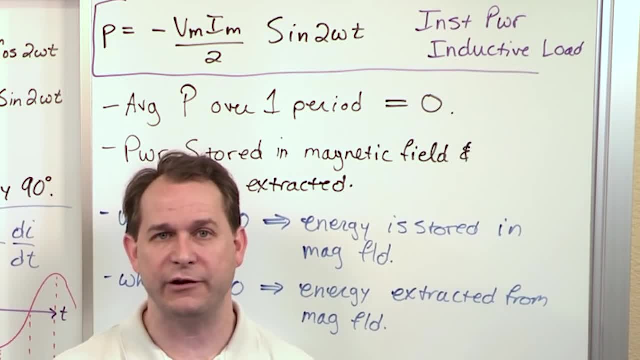 that the source is delivering is always negative, And we always said, hey, conservation of energy, the power delivered by the source is equal to the power that's dissipated or absorbed by the resistive network. right, So they have to add up. 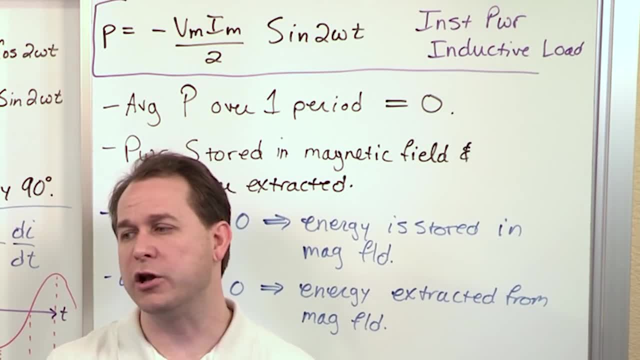 they have to be equal and opposite. So we've had the sign convention all along. Positive means the thing is absorbing something Negative. we've usually talked about negative power being sources. that's delivering power to the circuit. It's the same convention here. 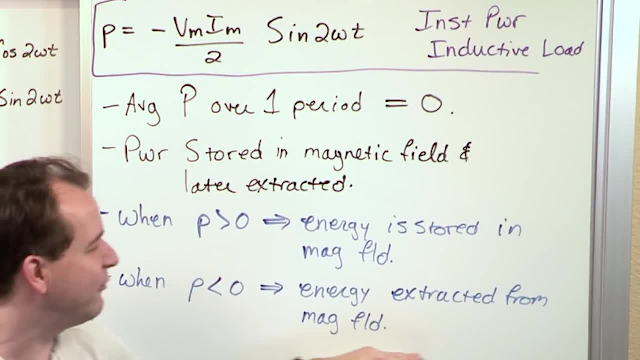 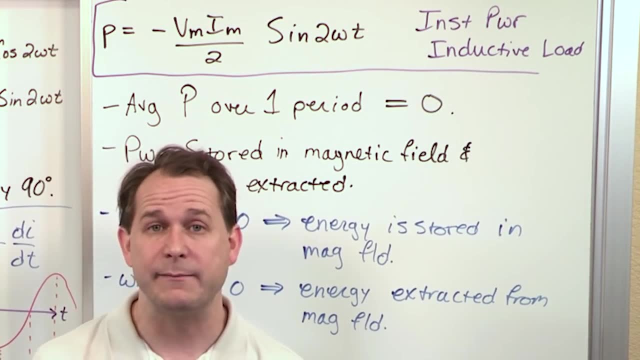 When the inductor is on the part of the cycle, where the inductor has negative power, it's just delivering energy much like a source, much like a temporary source of energy. In fact, it is because it's had energy stored in its magnetic field. 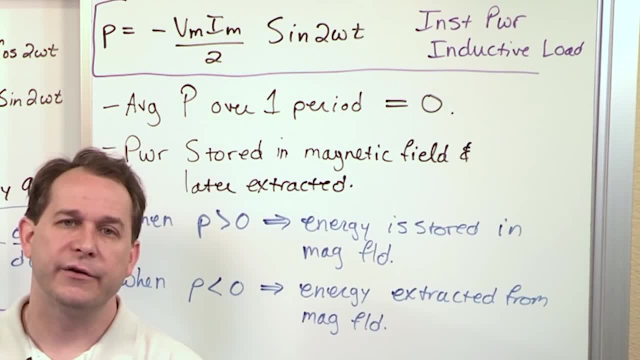 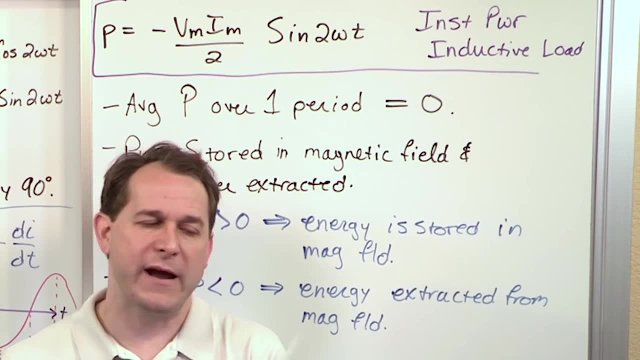 So the way to think about it is inductors and capacitors- we'll talk about here in the next section. when you get into these AC analysis cases, basically you have this sloshing around of energy sloshing, or you can think of it as like two buckets. 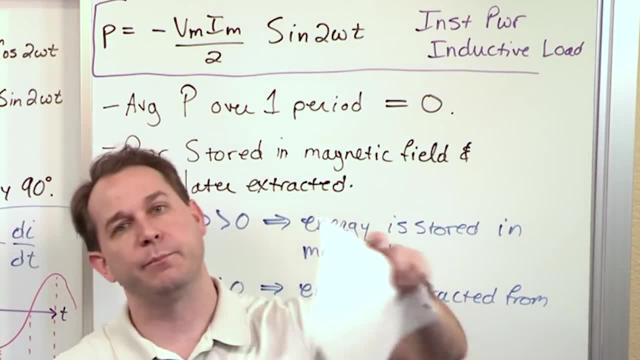 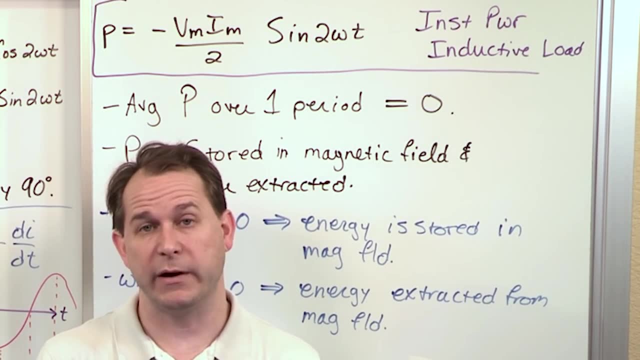 I'm pouring water in this bucket and pouring water in that bucket, pouring water in this bucket, pouring water in that bucket. On the whole, I'm not really. I don't really have any average power delivered anywhere on the whole, because half the time I'm pouring water in this bucket. 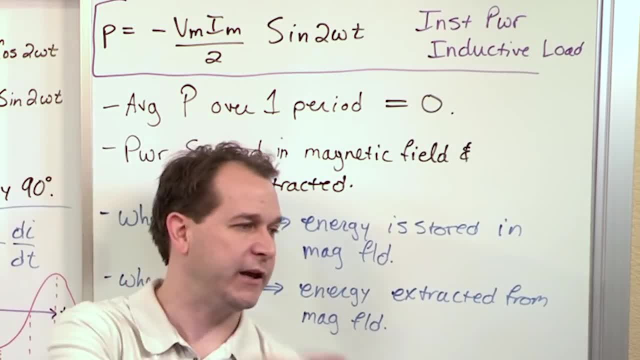 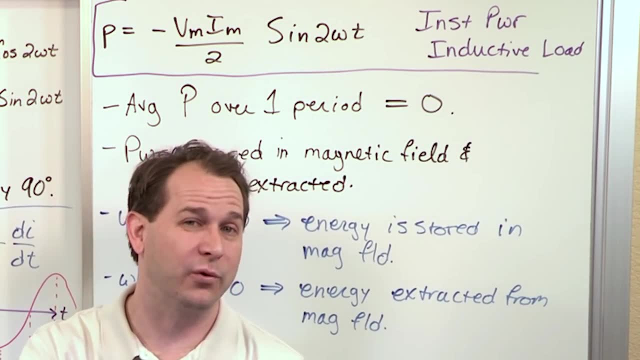 and half the time I'm pouring water in this bucket, So the water is just kind of staying here in my two hands. It's not going anywhere. That's why the average power is always zero, because half the time the inductor is absorbing energy. 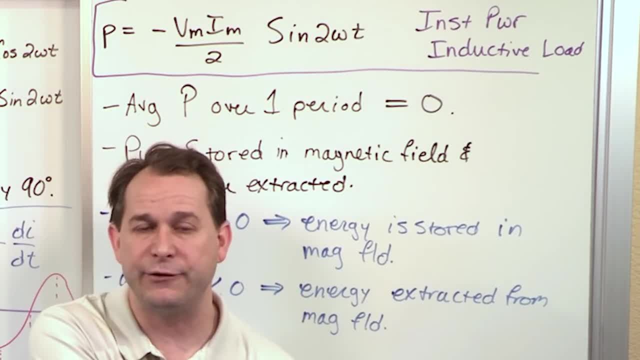 and the other half the time it's delivering energy back to the circuit that gave it the energy to begin with. So it's like this ping pong. I can use as many analogies as you want. It's like ping pong. I hit the ball this way, I hit the ball that way. 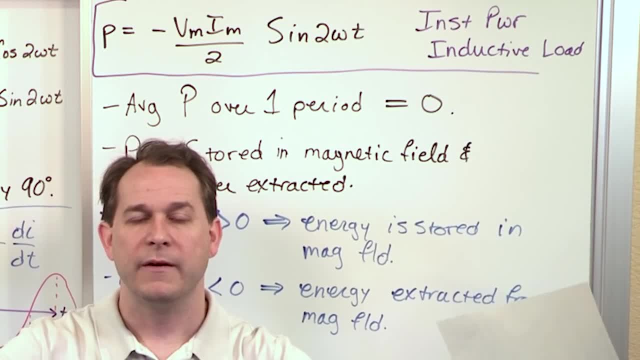 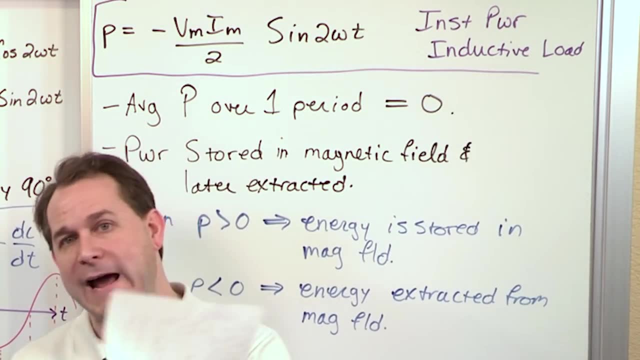 hit the ball this way. The ball's still staying here on this table, So average power is not really being radiated to the environment or anything. It's staying in the system. but half the time I'm delivering and half the time I'm absorbing. 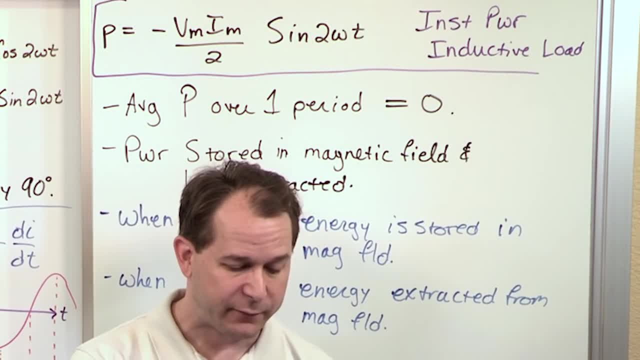 That's about as many analogies as I can give you there. but that's what's happening. Energy's sloshing around, It's sloshing back and forth, but the average power is zero over time because it's kind of always staying on the court here. 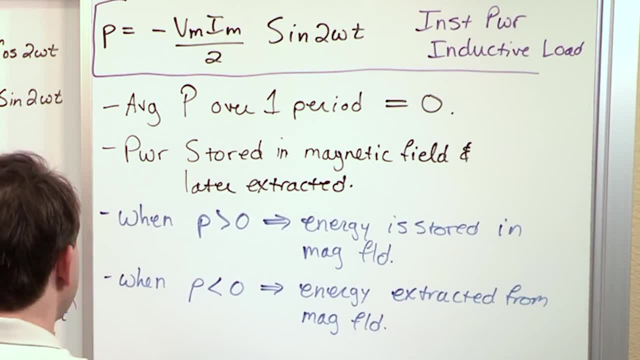 It's never going anywhere else. So the last thing I'm gonna leave you with is a little graph here. We said: this is the instantaneous power. This is what it is. Let's draw a picture of that real quick, and then we'll close the section off. 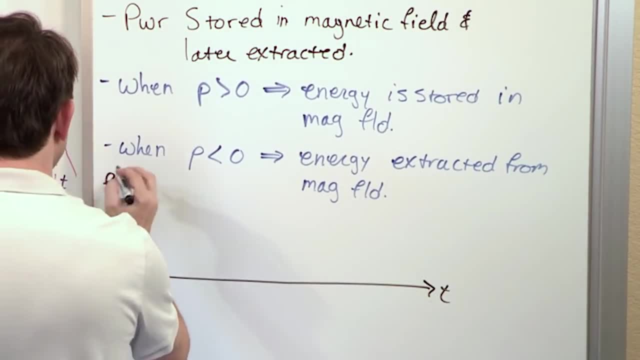 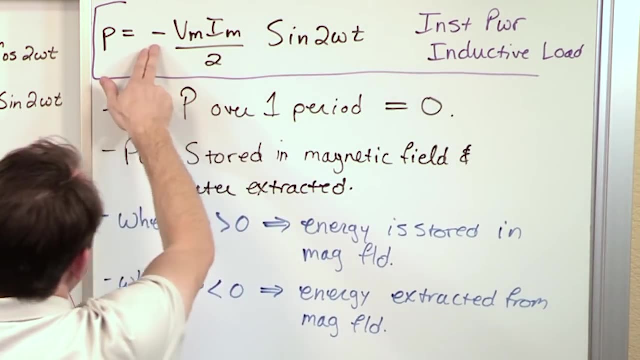 and talk about capacitors. So this is time. So this is the instantaneous power. What would this look like? Well, this is a constant, so forget about it. This is a sign. We know what signs look like, but we have a negative sign out there. 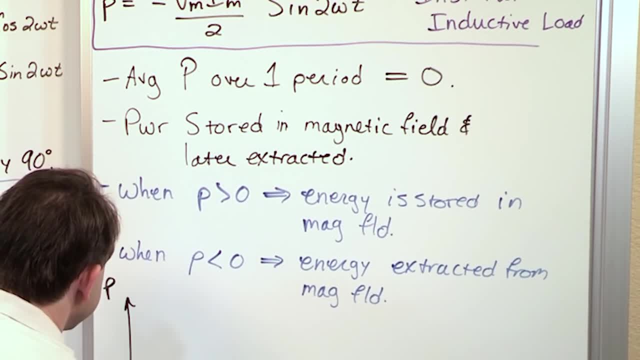 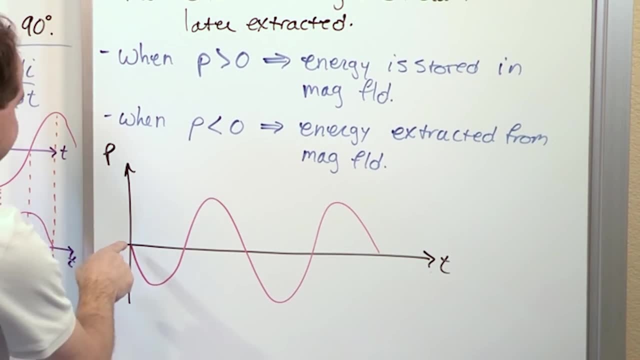 So it's gonna look like an upside down sign. It's gonna, instead of starting up like this, it's gonna start like this, Like this. okay, This is the instantaneous power. It starts in the negative direction only because of this negative sign. that's here. 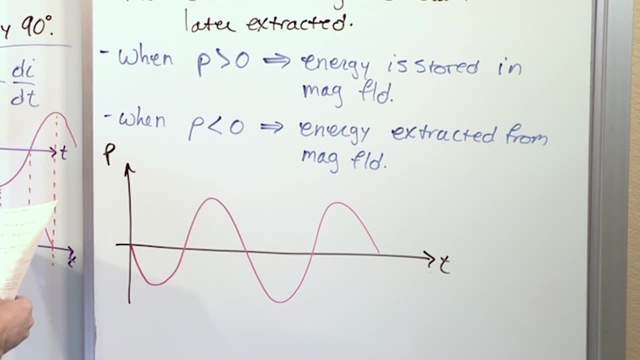 At time zero. that's what you have. And so it starts here, because it's negative. and you can see that initially it's negative, so the inductor's delivering energy, and then here it's absorbing and here it's delivering. 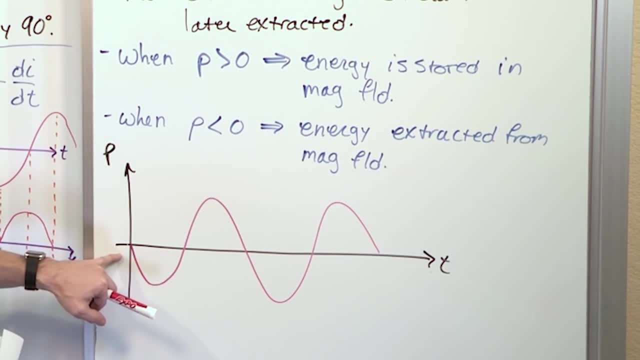 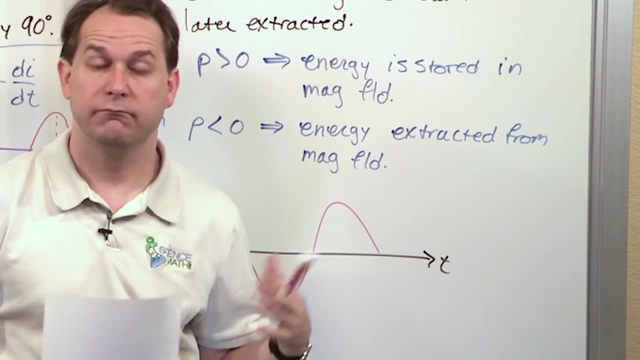 and here it's absorbing, and here it's delivering, and so on and so forth. I wanna draw a picture of this for you, because later on we talk about capacitors. This will be flipped upside down and it'll look the same, except it'll be upside down. 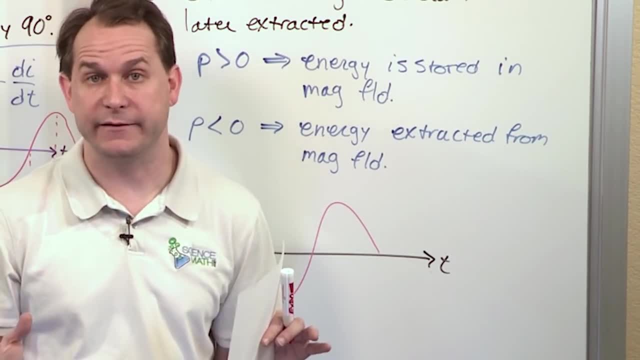 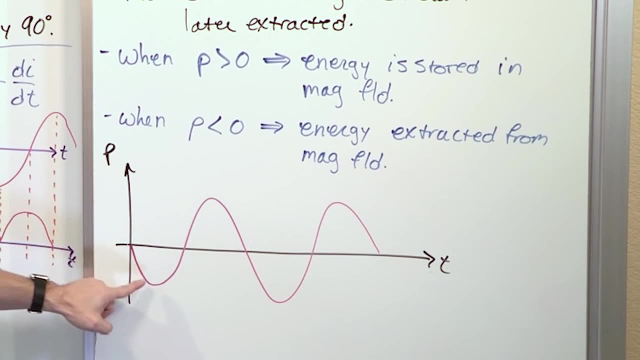 So I'm gonna be drawing a lot of parallels between inductors and capacitors as we go forward here. So the big takeaways and notice that the average power is zero. This is the instantaneous power, right, But if you draw a line right through the middle, 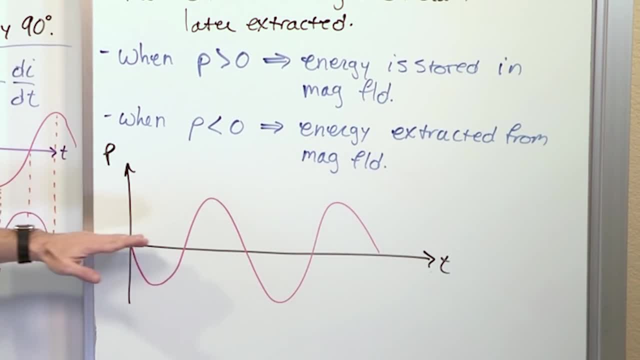 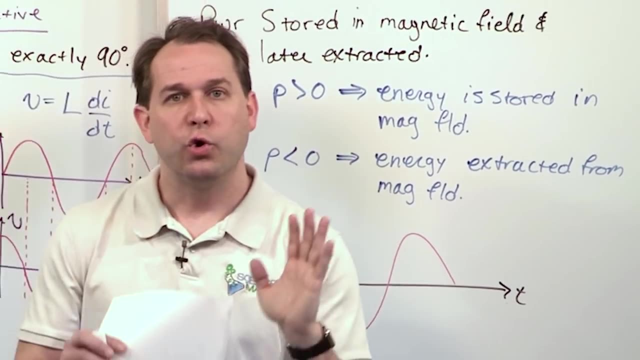 of course, you're just looking at the middle of the sine wave there. So the average power is zero half the time we're delivering and half the time we're absorbing power and this inductor. So quick, quick, 10 second recap. 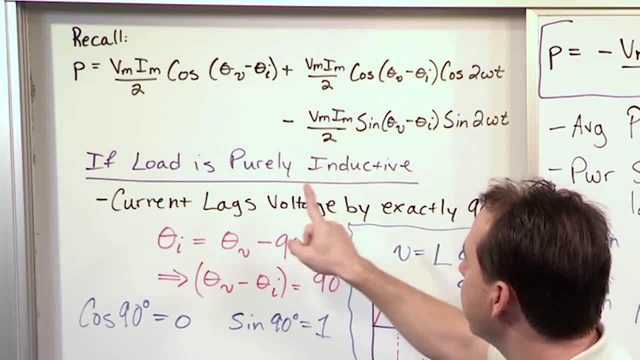 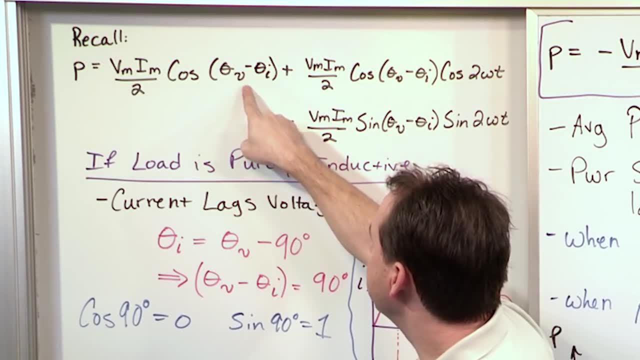 Here's the instantaneous power, the granddaddy equation. Then we figure out that for inductors, current lags, voltage, which means theta V minus theta I, is positive 90 degrees. We put 90 degrees in this term, this term disappears. 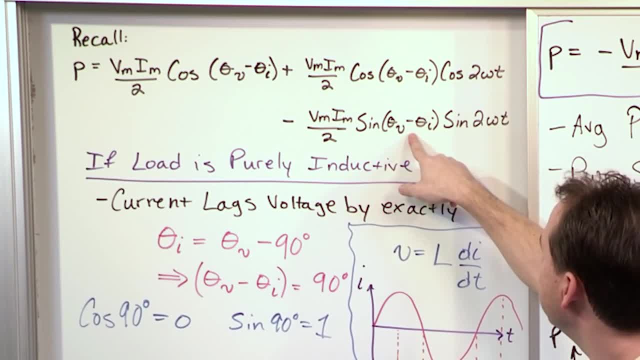 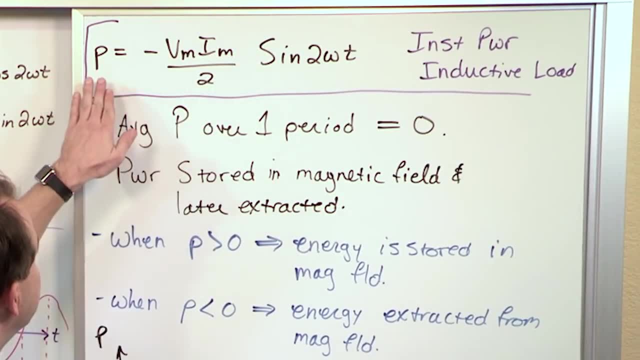 We put 90 degrees in this term, this term disappears. We put 90 degrees in this term and we're left with this times this, this is one, this whole thing's one times this, which is our instantaneous power equation for an inductive load. 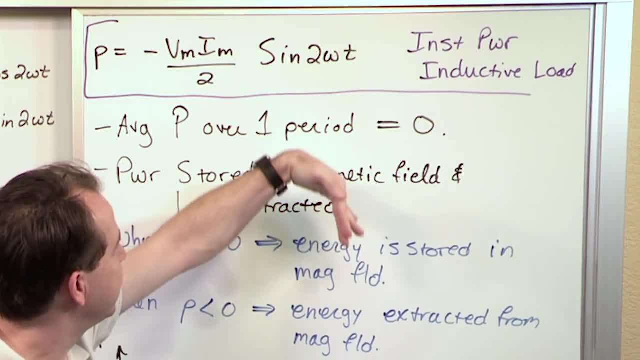 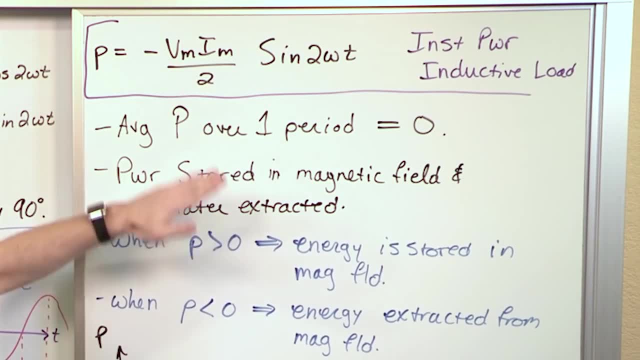 Because it's just a sign that it's half the time positive, half the time negative. the average power is zero, power stored in the magnetic field and later extracted. When this part of the cycle is positive, we're storing energy in the magnetic field. 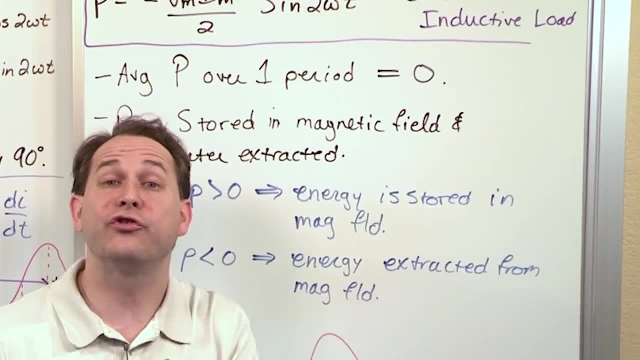 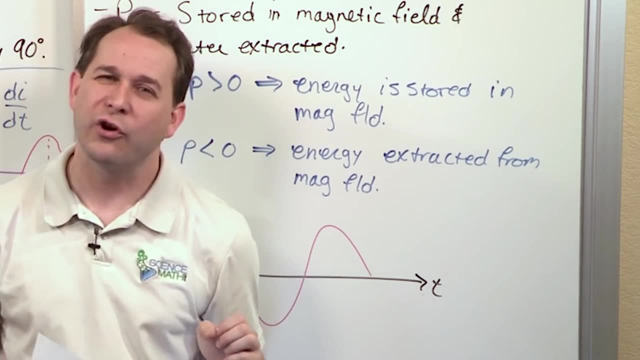 When the part of the cycle is negative, we're extracting energy and it's kind of sourcing from that inductor to the rest of the circuit- energy from the magnetic field. And here's a plot of what's going on. So try to internalize that as much as you can. 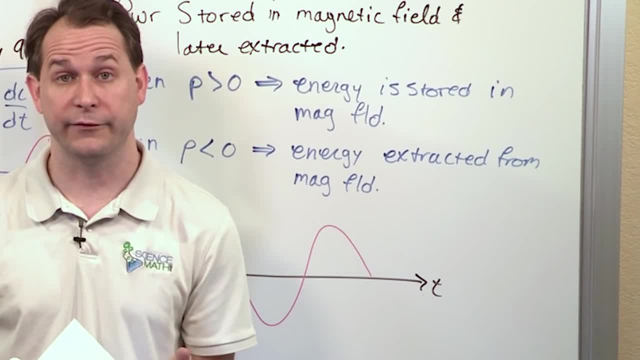 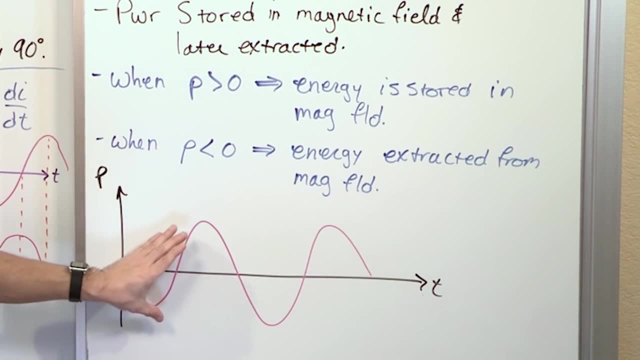 and relate that back to what we learned in the last section: for resistors. For resistors, the power like this was a sine wave, all right, but it did not have an average of zero. It was all shifted up and it was all positive up here. 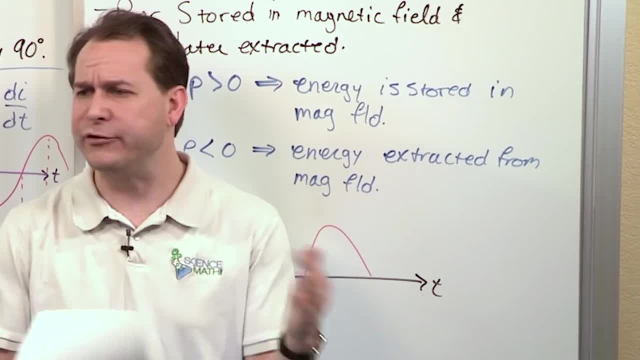 That's because resistors really do dissipate energy and you're not doing any sloshing. It can't store anything, So you can't slosh back and forth. You just deliver energy to that resistor and it gets radiated to the environment. 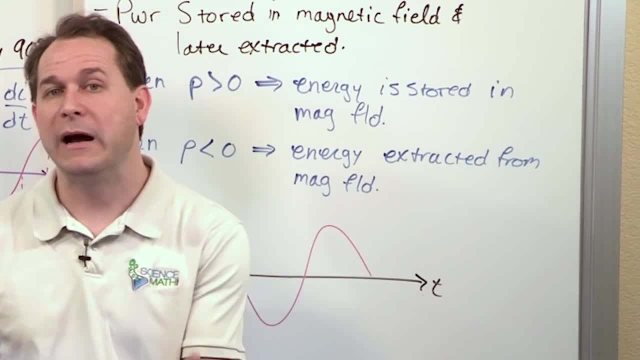 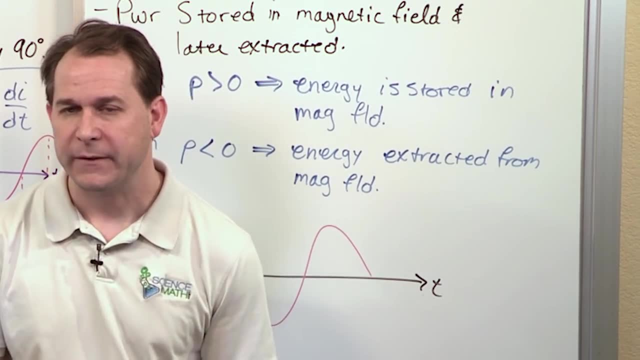 It's lost from the system. That's why the instantaneous power is always positive for resistors, But for inductors it can be positive and negative, depending on what part of the cycle you're at. So let me close here. Watch this a few times to get it. 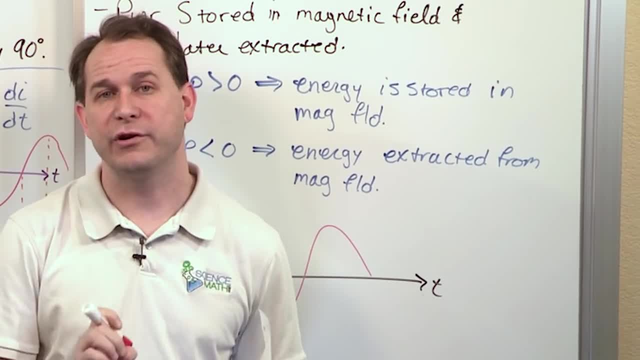 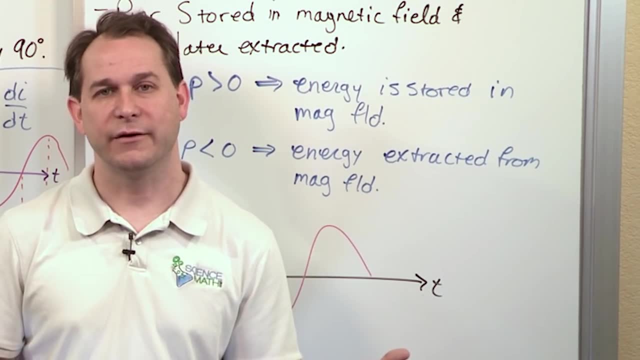 Follow me to the next section and we will make a very similar argument to show you how capacitors are very similar but yet obviously slightly different. It's the cousin to the inductor, So you'll see how that works in the next section.